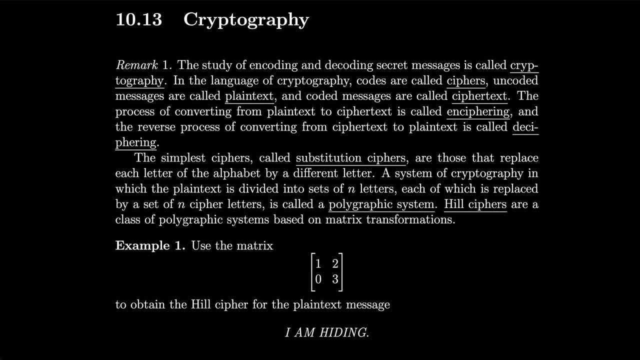 and the reverse process of converting from ciphertext to plaintext is called deciphering. The simplest ciphers, called substitution ciphers, are those that replace each letter of the alphabet by a different letter. A system of cryptography in which the plaintext is divided into sets of n letters, each of which is replaced by a set of n cipher letters, is called a. 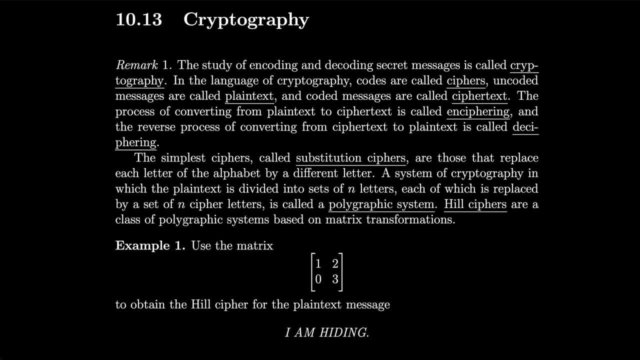 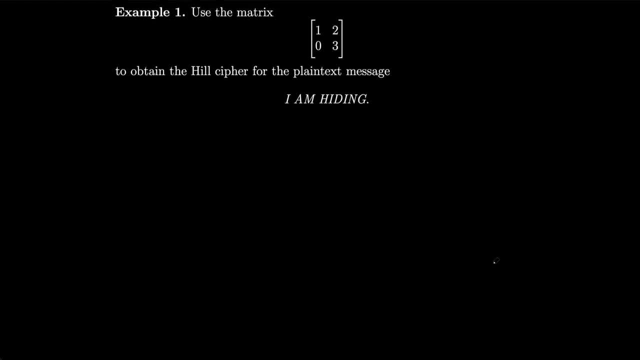 polygraphic system. Hill ciphers are a class of polygraphic systems based on matrix transformations. As an example, how about we use the matrix to obtain the hill cipher for the plaintext message I am hiding? So to obtain the hill cipher, we first group the letters that we want to. 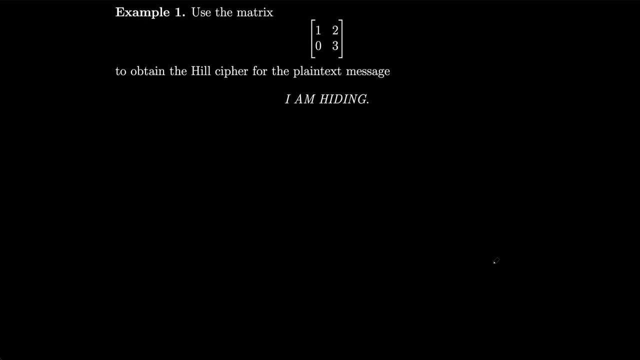 end up with. So I'll write i- a, and then I'll write m, h, i, d, i, n and g, g separately. So then i is the 9th letter of the alphabet, so I'll assign 9 to it. 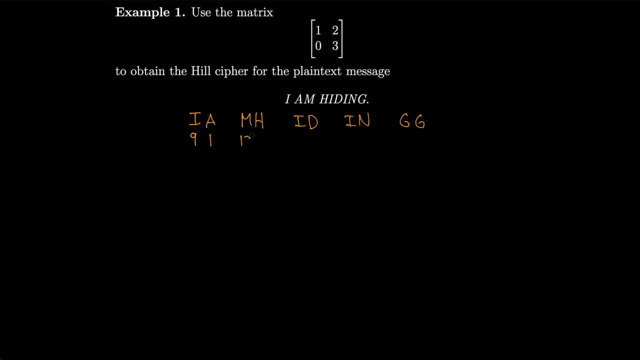 a is the 1st, so I assign 1,. n is the 13th, so I assign 13,. h is 8th, i is 9th. again d is 4th, i is 9th, n is 14th, g is 7.. 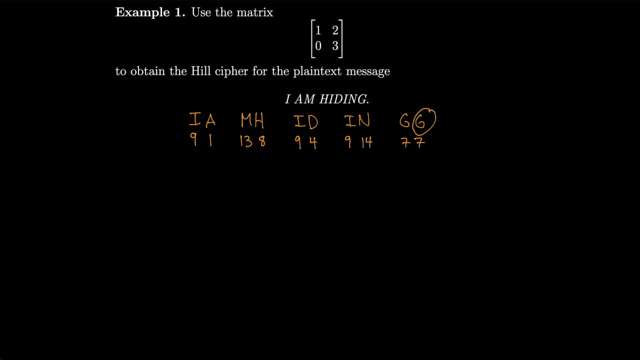 So notice, I put an extra g because I want to have an even number here, so I just duplicated the last letter. Okay, so now let's encode this, or cipher this, using matrices. So I'm going to use the matrix 1,, 2,, 0,, 3 and multiply it by each of these guys as matrices. 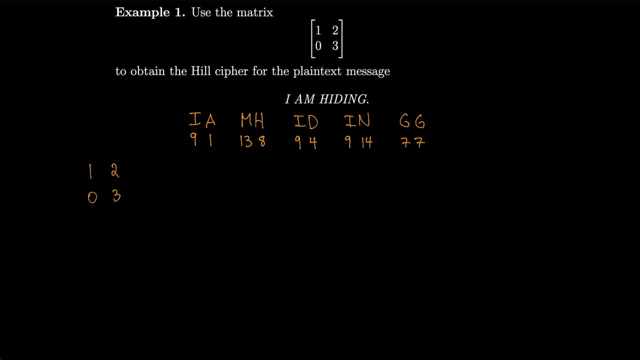 So I'll take 1,, 2,, 0,, 3 and multiply it by i, a, which is 9, 1,, so that I can get 11, 3.. And the 11th letter of the alphabet is k, the 3rd is c, so that gives me kc. 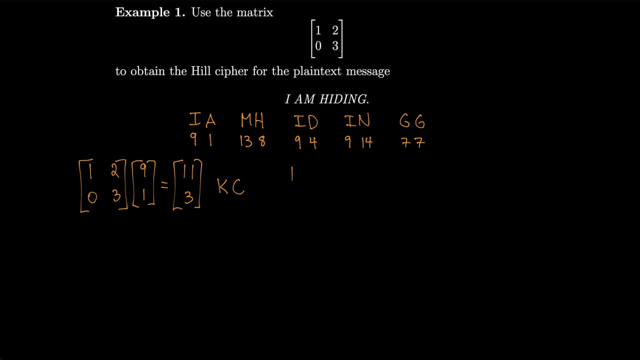 Okay, next I will take 1,, 2,, 0,, 3 and multiply by 13, 8 for m h and I'll get 29, 24.. 29 is too far in the alphabet, so I just basically keep going loop back around. 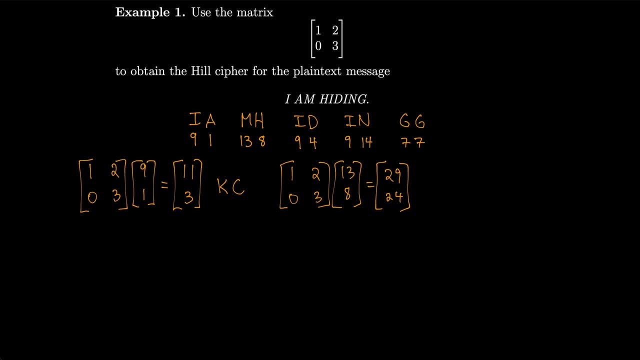 It's 3 past the last letter, so I'll replace that with 3, 24, and I'll get c for 3 and x for 24.. So then let's keep going. 1,, 2,, 0, 3 times 9, 4 gives me 17,, 12.. 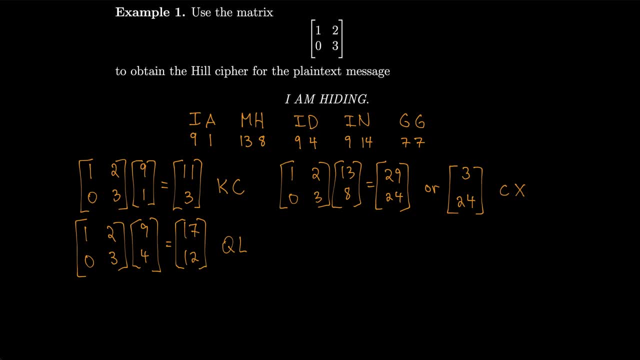 So that's q? l. Then 1,, 2,, 0,, 3 times 9,, 14 gives me 37,, 42. And again, that's past the 26 letter of the alphabet. So I see how far past 26 I am for each of them. And it's 11 for 37 and 16 for 12.. So that's q, l. Then 1,, 2,, 0,, 3 times 9,, 14 gives me 37,, 42. And again, that's past the 26 letter of the alphabet. 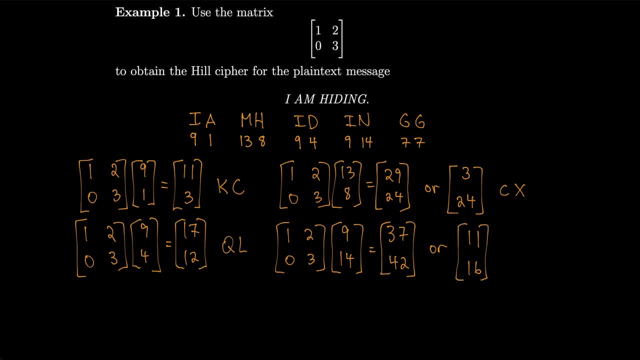 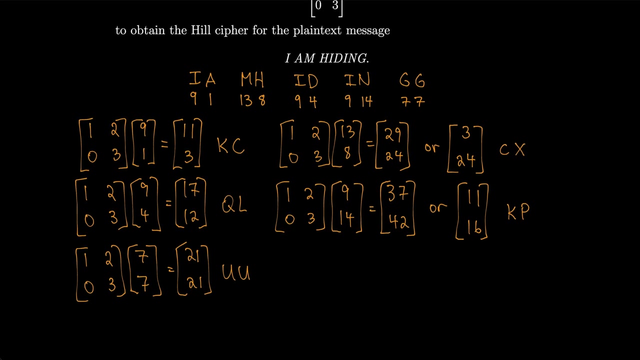 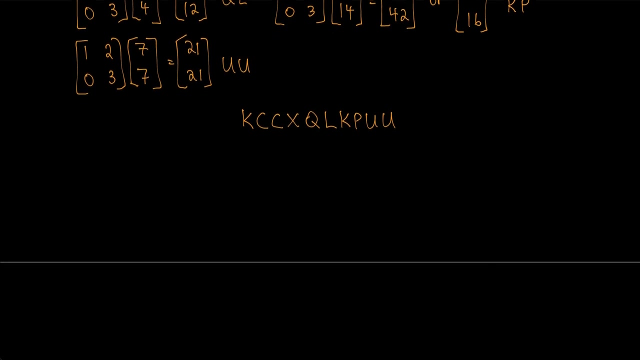 16 for 42, so I'll take kp. And then, lastly, 1203 times 77 gives me 2121, which is uu. So altogether- I am hiding under the Hill cipher- becomes k, c, c, x, q, l, k, p, u, u. 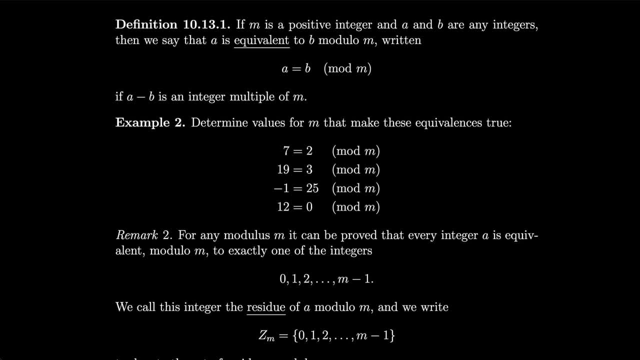 If m is a positive integer and a and b are any integers, then we say that a is equivalent to b modulo m. written a equals b mod m if a minus b is an integer multiple of m. That's basically what we were doing over here when we were reducing these guys over. 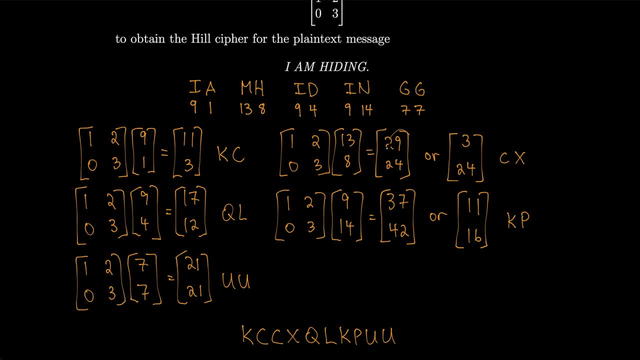 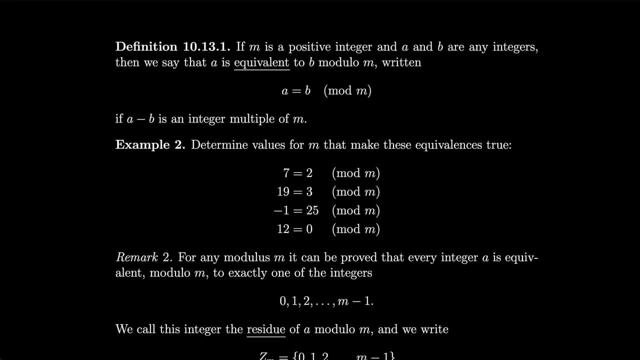 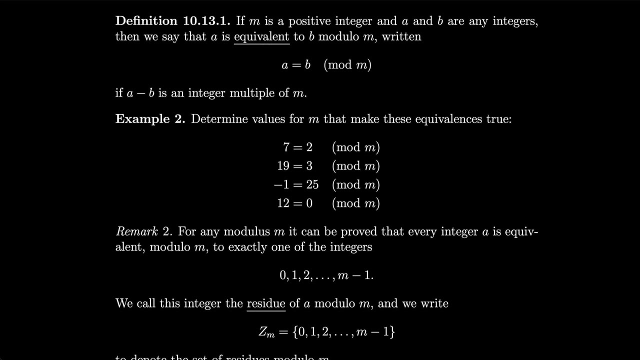 here because they were basically the numbers we got were too big, so we essentially divided by 26 and got the remainder. So let's determine values for m that make these equivalences true. So let's see, what do we? what could we take to have 7 equal to 2 mod m? 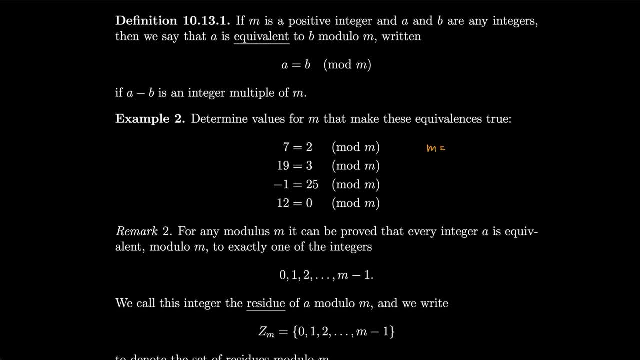 Well, if we make m equal to 2 mod m, that's going to be 0.. If m equals 5, then 7 minus 2 will be a multiple of 5, because it would be exactly 5.. For the second one, 19 minus 3 would be 16.. 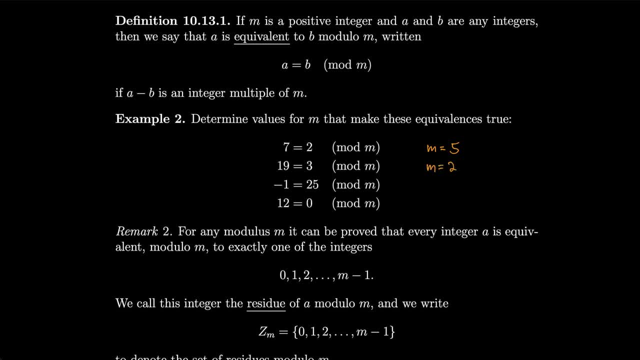 16 is a multiple of 2, so we could take: m equals 2.. For the next one we could do, let's see: negative 1 minus 25 would be negative 26,, which is a multiple of 26.. 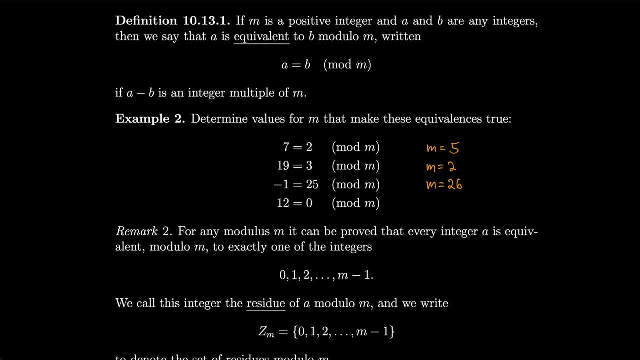 So we could just take m equals 2.. And then for the last one, 12 minus 0 is 12,, which is a multiple of 4, so we could take m equals 4.. Obviously, these are not the only values that would work. it could have just said: take. 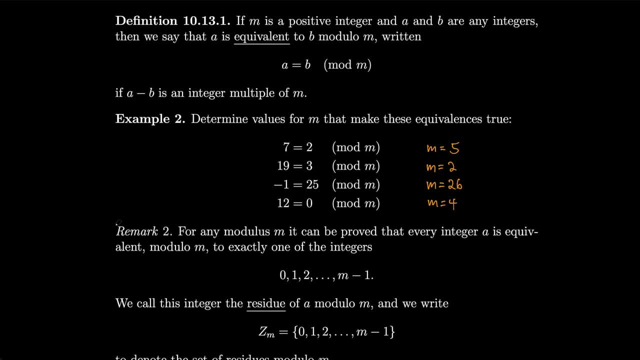 m equals 12, and that would still have worked For any modulus m. it can be proved that every integer a is equivalent modulo m to exactly one of the integers from 0 to m minus 1.. We call this integer the residue of a modulo m. 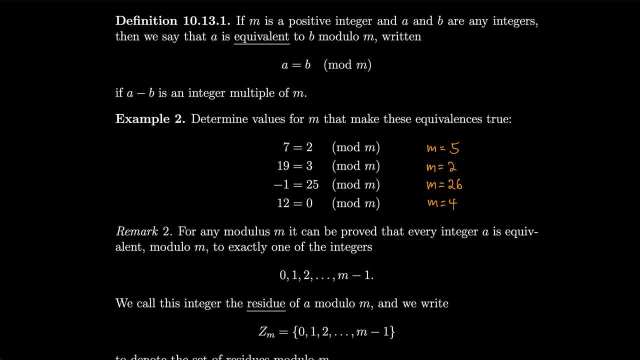 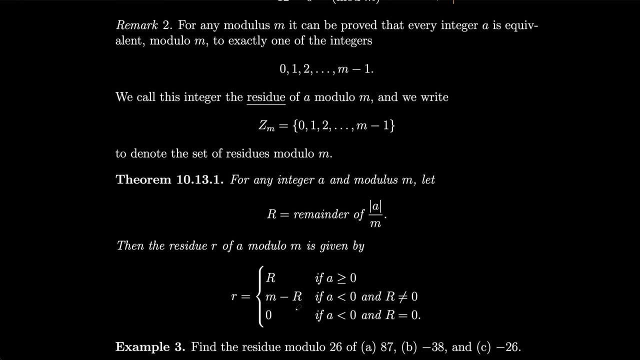 And we write: Zm is the set of the integers from 0 to m minus 1 to denote the set of residues, modulo m For any integer a and modulus m. let r equal the remainder of the absolute value of a divided by m. 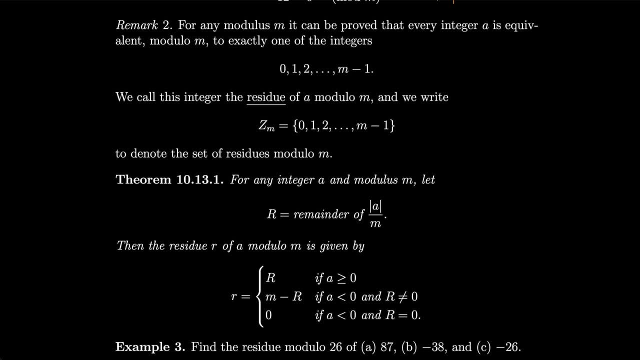 So then the residue r of a modulo m is given by capital R, if a is greater than or equal to 0.. So it's the remainder. if a is positive, It's m minus 0.. m minus r if a is negative and the remainder is not 0. 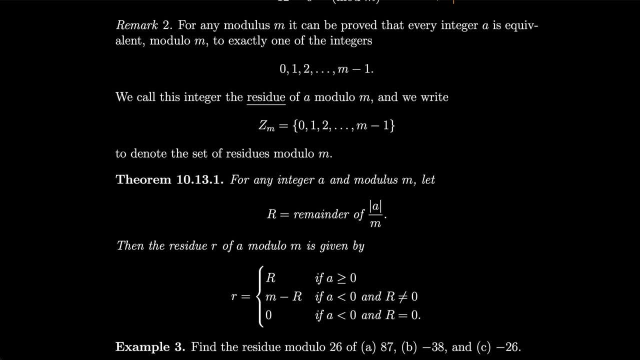 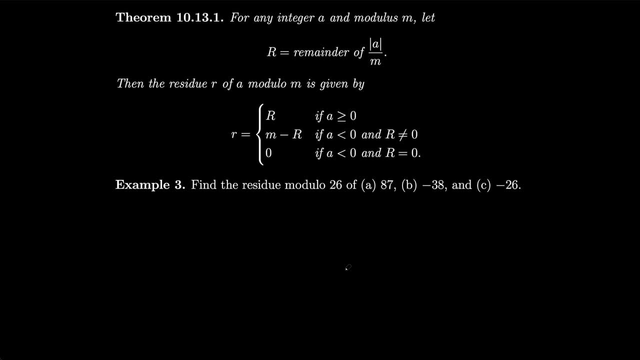 And it's 0 if a is negative and the remainder is 0.. Let's find the residue modulo 26 of 87, negative 38, and negative 26.. So for a we have that r is equal to the remainder of. 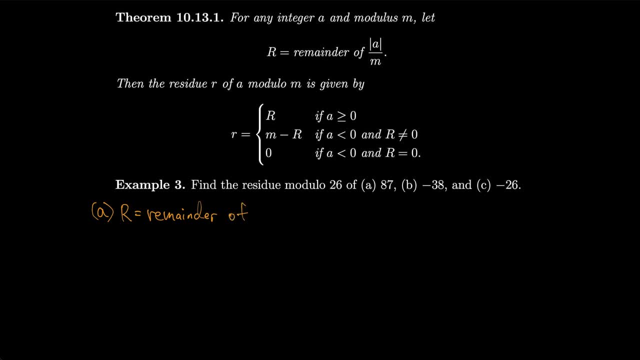 Let's see. so what we have to do is take the absolute value of a, so that's the absolute value of 87, and then divide that by m, which is 26, because i said modulo 26, so that gives me 9, because it's the remainder of 87 divided by 26. it'd be 9 left over if i divide 87 by 26, and 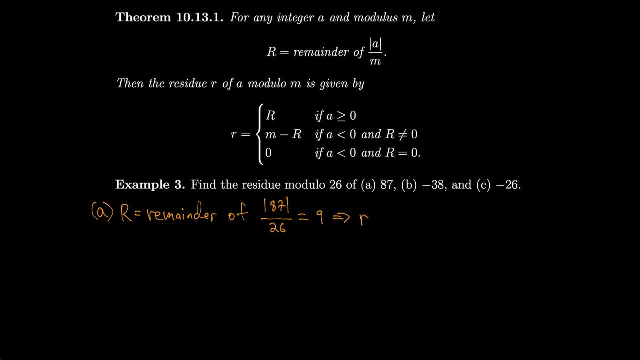 that gives me the residue is 9. okay, how, so that means that i could write: 87 is equal to 9 modulo 26. for b, let's do r- is equal to the remainder of negative 38 over 26. take the absolute value, so that would be. you can think of it almost like. 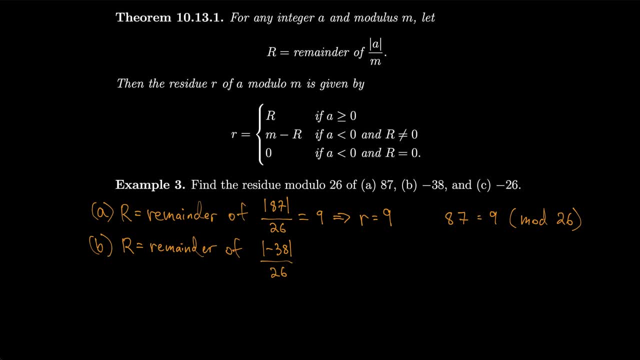 a mixed number. in this case, that's 1 and 12, 26. so the remainder is 12. so we have r in this case, because our a was negative. so we have r in this case, because our a was negative, little r. the residue is m minus r, so it's 26 minus 12, which is 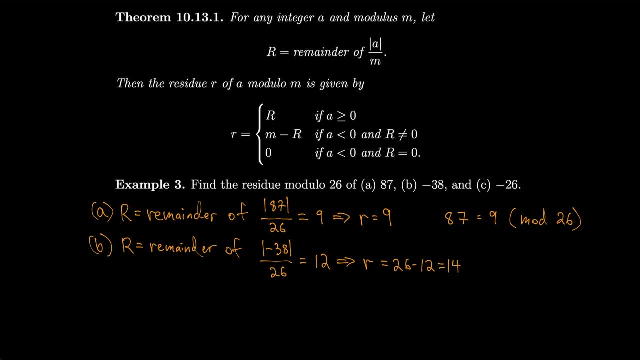 14. so we have negative 38 equals 14 modulo 26.. okay, let's do c, so we have r. is okay, let's do c, so we have r. is okay, let's do c, so we have r. is the remainder of absolute value negative 26 over 26. 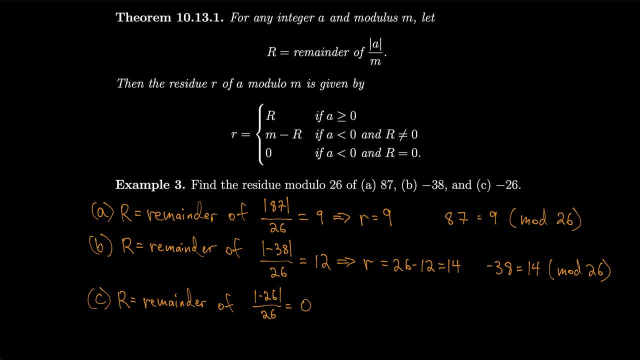 and that remainder is zero, because 26 fits perfect. negative 26 fits perfectly in there. so that means that r is equal to zero and that means that we have negative 26 is equal to zero and that means that we have negative 26 is equal to zero. 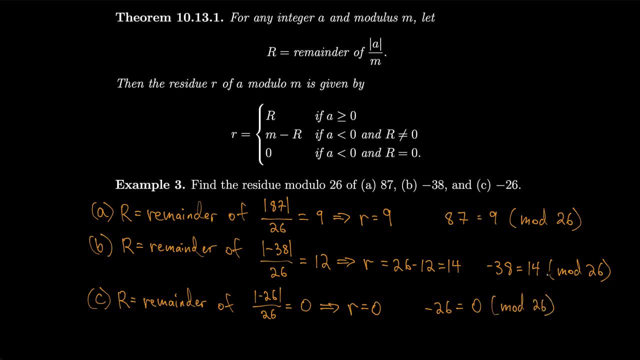 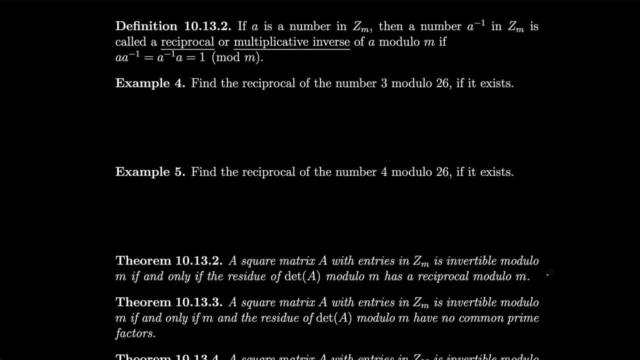 modulo 26. if a is a number in zm, then a number a inverse in zm is called a reciprocal or. modulo 26 is called a reciprocal or multiplicative inverse of a modulo m. multiplicative inverse of a modulo m. multiplicative inverse of a modulo m. if a a inverse is equal to a inverse a. 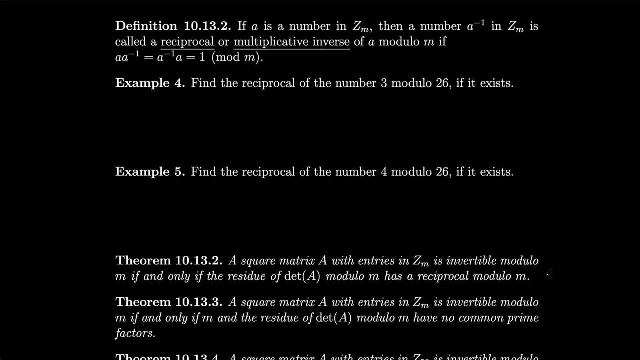 if a, a inverse is equal to a inverse a. if a, a inverse is equal to a inverse a, which is equal to 1 modulo m, which is equal to 1 modulo m, which is equal to 1 modulo m. let's find the reciprocal of the number. 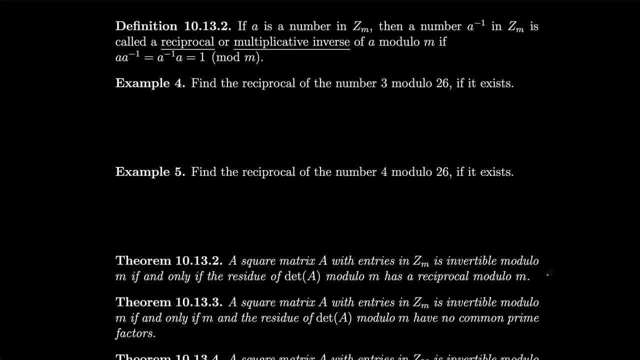 let's find the reciprocal of the number. let's find the reciprocal of the number 3 modulo 26, if it exists. 3 modulo 26 if it exists. 3 modulo 26, if it exists. so what we'll do is we'll set 3x. 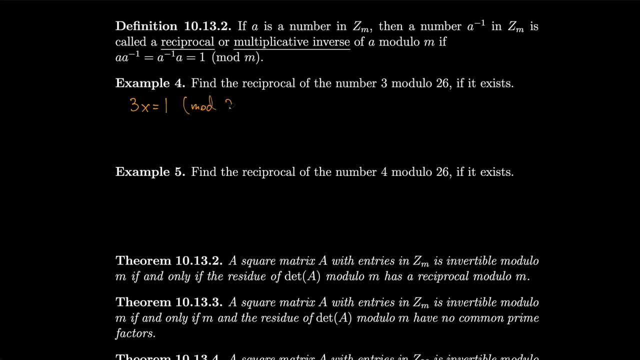 so what we'll do is we'll set 3x. so what we'll do is we'll set 3x equal to 1 modulo 26, equal to 1 modulo 26, equal to 1 modulo 26, and we'll just keep trying numbers and 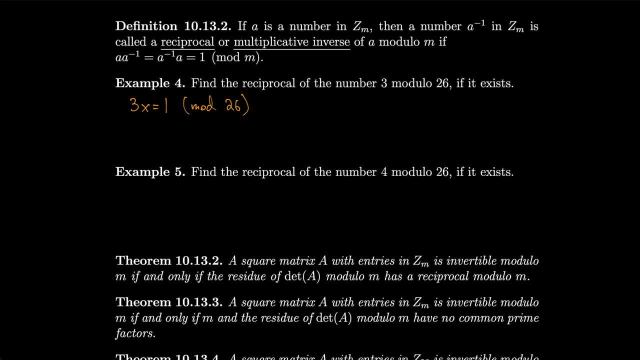 and we'll just keep trying numbers, and, and we'll just keep trying numbers and plugging them in until we get uh, plugging them in until we get uh, plugging them in until we get uh, something that hopefully works as the, something that hopefully works as the. 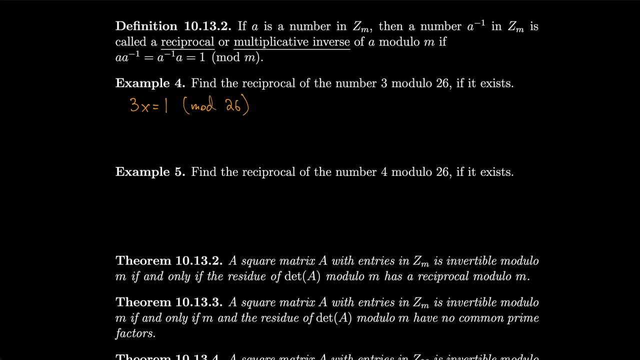 something that hopefully works as the inverse, inverse, inverse. so we'll try 0, 1, 2, 3, 4, 5, etc. all the. so we'll try 0, 1, 2, 3, 4, 5, etc. all the. so we'll try 0, 1, 2, 3, 4, 5, etc. all the way up through 26. way up through 26. way up through 26. i'm not going to write all of them, but it i'm not going to write all of them, but it i'm not going to write all of them, but it turns out that if you try turns out that if you try. 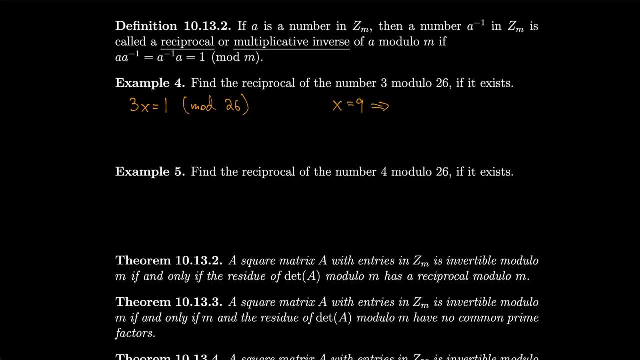 turns out that if you try x equals 9, then you get x equals 9, then you get x equals 9, then you get 3 times 9, which is 27, and 27 is actually 1. 27 and 27 is actually 1. 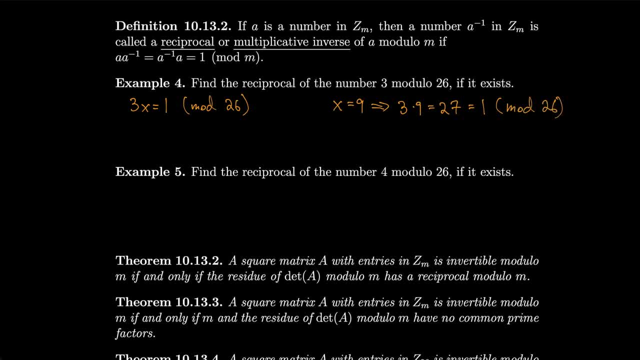 27 and 27 is actually 1 modulo 26, right? because if you take 27 modulo 26, right? because if you take 27 modulo 26, right? because if you take 27 divided by 26, the remainder is divided by 26. the remainder is: 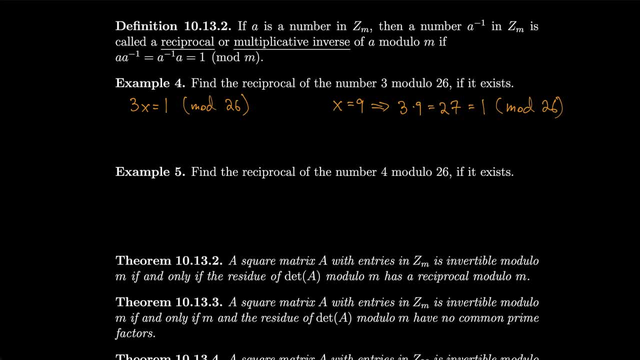 divided by 26, the remainder is 1. beautiful, so that means that: 1. beautiful, so that means that 1. beautiful, so that means that 3 inverse is equal to 9, 3 inverse is equal to 9, 3 inverse is equal to 9 modulo 26. 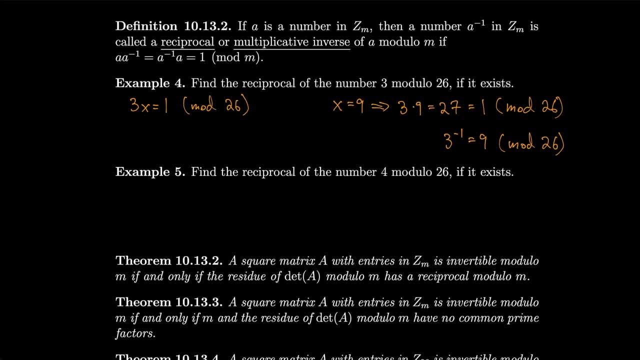 so yeah, it could take a long time to. so yeah, it could take a long time to. so yeah, it could take a long time to find the reciprocal, find the reciprocal, find the reciprocal, because you've tried a lot of numbers, because you've tried a lot of numbers. 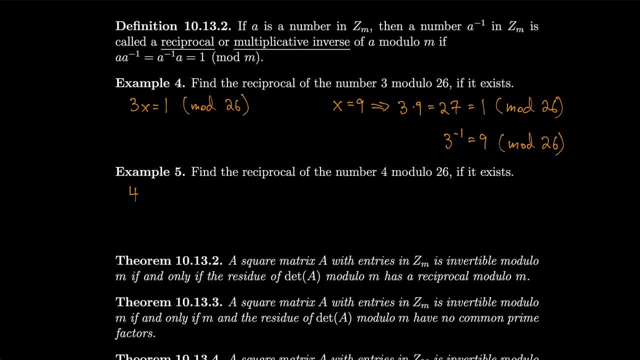 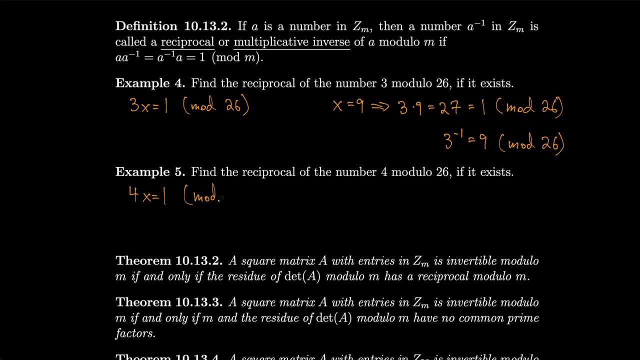 number 4 modulo 26, if it exists. number 4 modulo 26, if it exists, so we'll set 4 x equal to 1, so we'll set 4 x equal to 1, so we'll set 4 x equal to 1 mod 26, and we'll try 0 through 25. 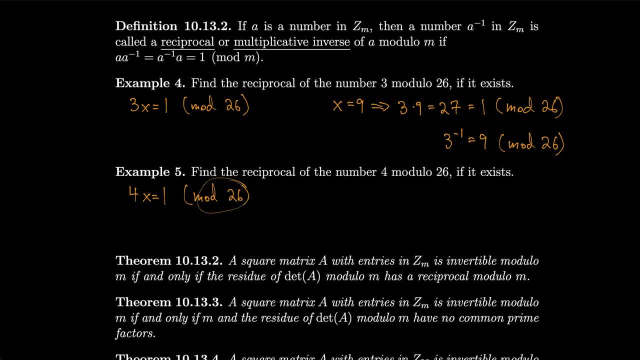 mod 26, and we'll try 0 through 25 mod 26 and we'll try 0 through 25 again. because we're trying all the again, because we're trying all the again, because we're trying all the numbers up until 26, numbers up until 26. 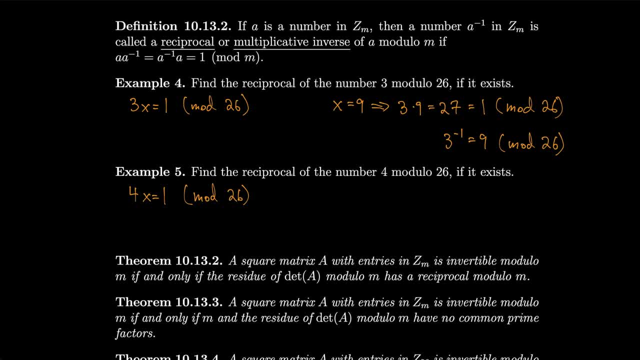 numbers up until 26, and it turns out that, uh, and it turns out that, uh, and it turns out that, uh, we won't get any reciprocal. but this, we won't get any reciprocal. but this, we won't get any reciprocal. but this kind of makes sense because 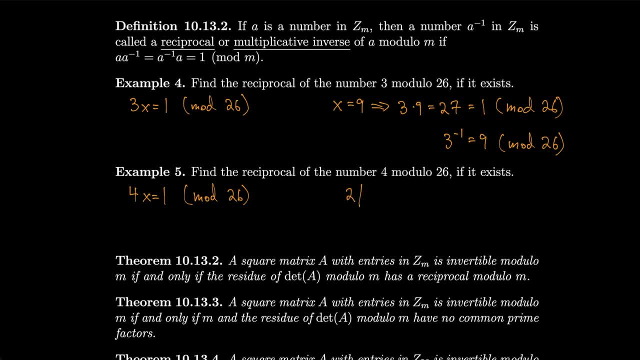 kind of makes sense. because. because kind of makes sense? because two divides four, two divides four, two divides four. let me write it like this for divides. let me write it like this for divides. let me write it like this for divides and and and two also divides 26.. 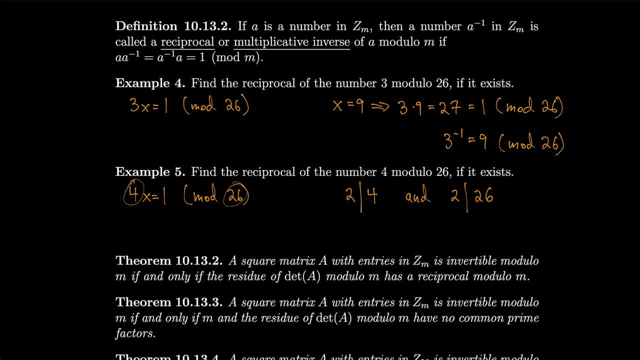 two also divides 26.. two also divides 26.. so so so four and six, four and six, four and six. both share a common divisor of two. both share a common divisor of two. both share a common divisor of two. so that should tell you that there won't. 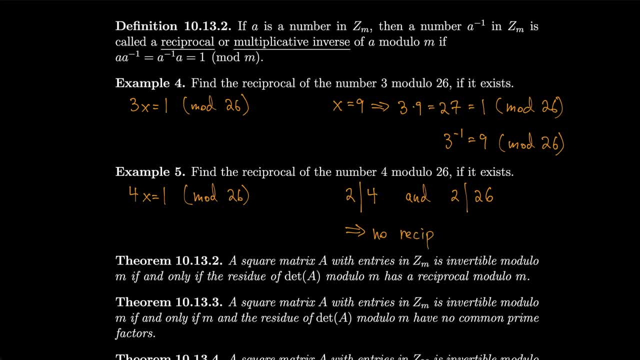 so that should tell you that there won't. so that should tell you that there won't be any reciprocal, because it's divisible, because it's divisible, because it's divisible. any square matrix a with entries in zm is. any square matrix a with entries in zm is: 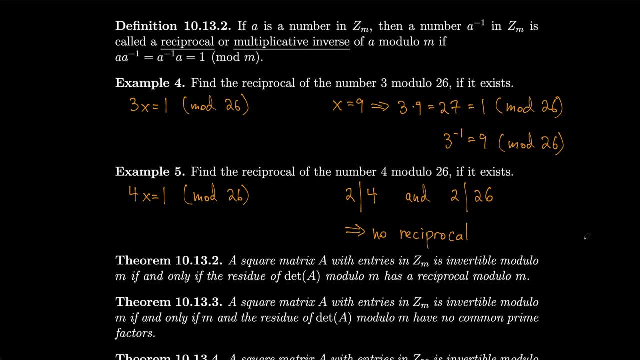 any square matrix a with entries in zm is invertible modulo m if and only if the invertible modulo m, if and only if the invertible modulo m, if and only if the residue of the determinant a modulo m, residue of the determinant a modulo m, residue of the determinant a modulo m, has a reciprocal modulo m. so that's why. 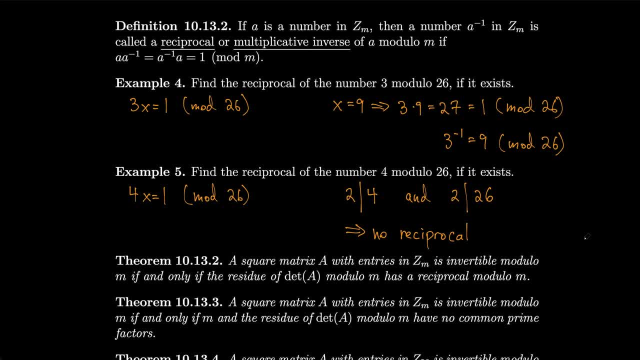 has a reciprocal modulo m. so that's why has a reciprocal modulo m. so that's why we care about reciprocals a square. we care about reciprocals a square. we care about reciprocals a square. matrix a with entries in cm is. matrix a with entries in cm is: 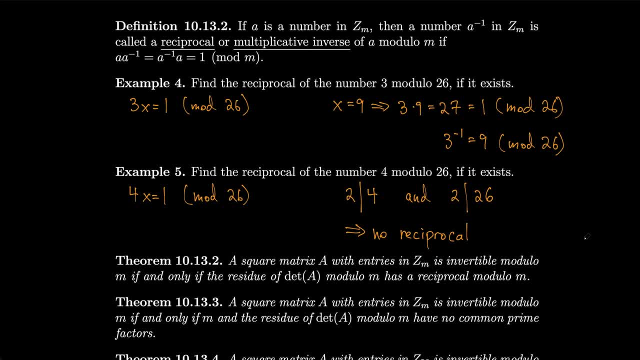 matrix a with entries in cm, is invertible modulo m. if and only if invertible modulo m. if and only if invertible modulo m. if and only if the residue of determinant modulo m, the residue of determinant modulo m, the residue of determinant modulo m have no common prime factors. 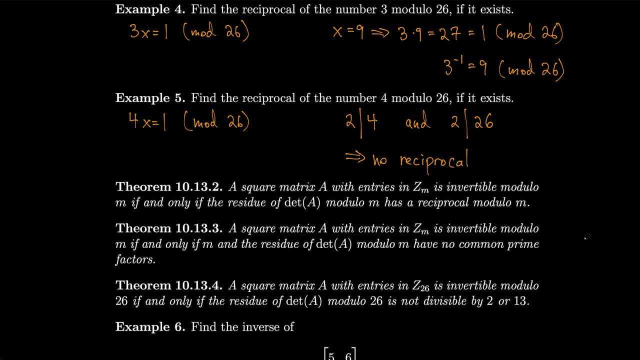 have no common prime factors. have no common prime factors. so m and the residue of determinant a. so m and the residue of determinant a. so m and the residue of determinant a have to have no common factors. have to have no common factors. have to have no common factors. a square matrix a with entries in z26. 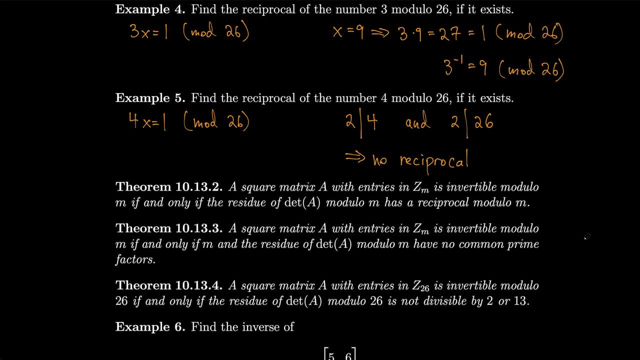 a square matrix a with entries in z26. a square matrix a with entries in z26 is invertible modulo 26. if and only if is invertible modulo 26. if and only if is invertible modulo 26. if and only if the residue of determinant a modulo 26. 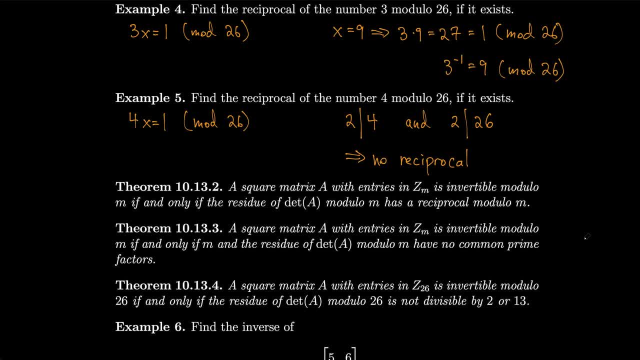 the residue of determinant a modulo 26. the residue of determinant a modulo 26 is not divisible by 2 or 13, is not divisible by 2 or 13. is not divisible by 2 or 13. as we can see over here, it was divisible. 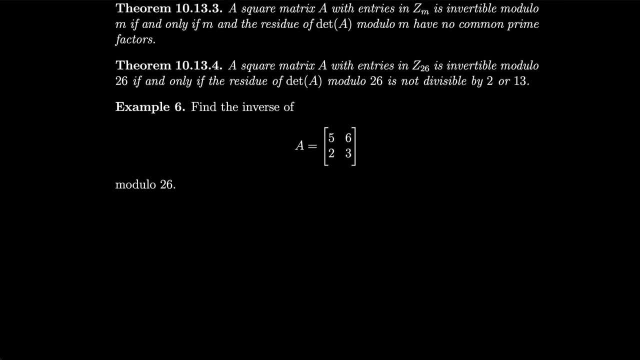 as we can see over here, it was divisible. as we can see over here, it was divisible by 2, so we got no reciprocal by 2. so we got no reciprocal by 2, so we got no reciprocal. let's find the inverse of uh this. let's find the inverse of uh this. 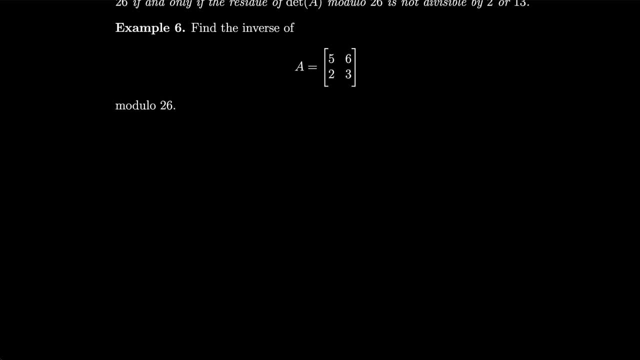 let's find the inverse of, uh, this matrix, a modulo 26 matrix, a modulo 26 matrix, a modulo 26. so, as we've seen previously, we can find. so, as we've seen previously, we can find. so, as we've seen previously, we can find the inverse of a two by two matrix. 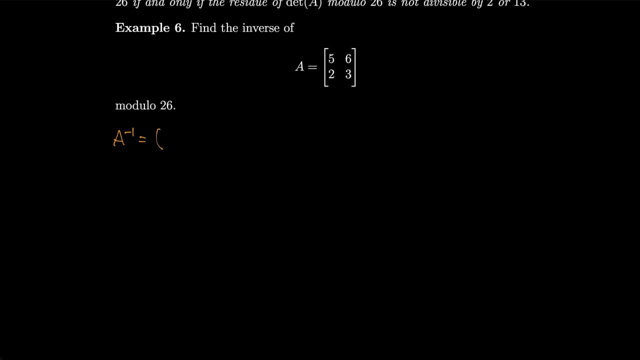 the inverse of a two by two matrix. the inverse of a two by two matrix, by taking one over the determinant. so by taking one over the determinant, so by taking one over the determinant. so that would be, that would be. that would be a d minus b c inverse, or 1 over a d. a d minus b c inverse, or 1 over a d. a d minus b c, inverse, or 1 over a d minus b c, minus b c times. well, we switch a and d, so we minus b c times. well, we switch a and d, so we. 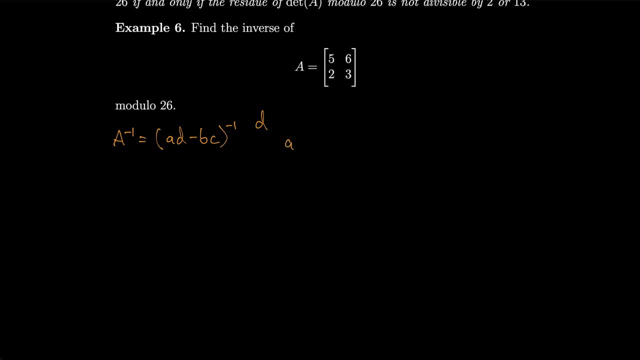 minus b c times. well, we switch a and d, so we get d get, d, get d a, and then we make b and c a, and then we make b and c a, and then we make b and c negative, negative, negative. in this case, we have to take everything. 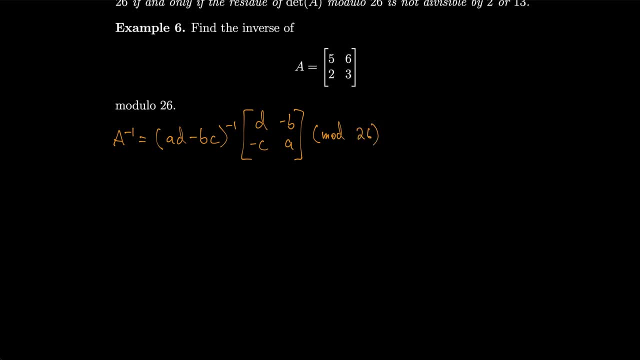 in this case, we have to take everything. in this case, we have to take everything. mod 26, though: okay, so let's get the determinant of a. okay, so let's get the determinant of a. okay, so let's get the determinant of a. so determinant of a. 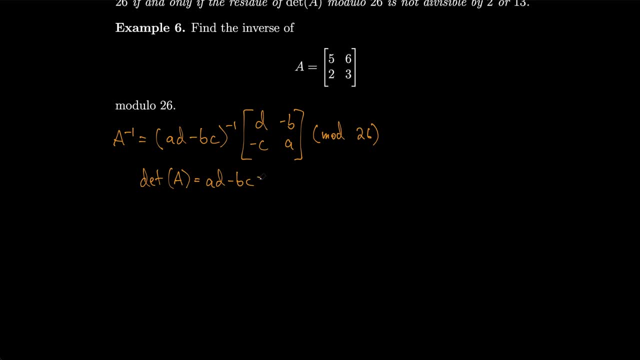 so determinant of a, so determinant of a is a, d is a, d is a d minus b c. so that's five times three minus b c. so that's five times three minus b c. so that's five times three minus six times two, which is three. 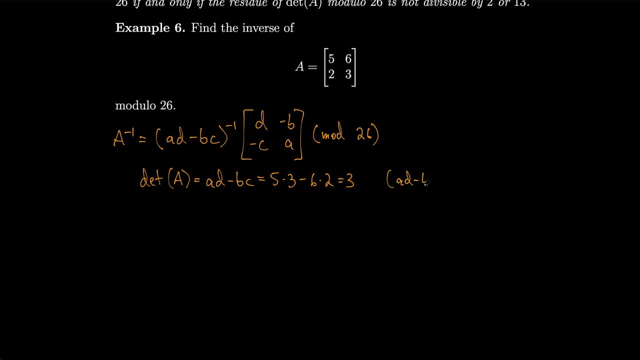 minus six times two, which is three, minus six times two, which is three. so that means that uh a d. so that means that uh a d. so that means that uh a d minus b c inverse. minus b c inverse. minus b c inverse. well, that'll be three inverse. 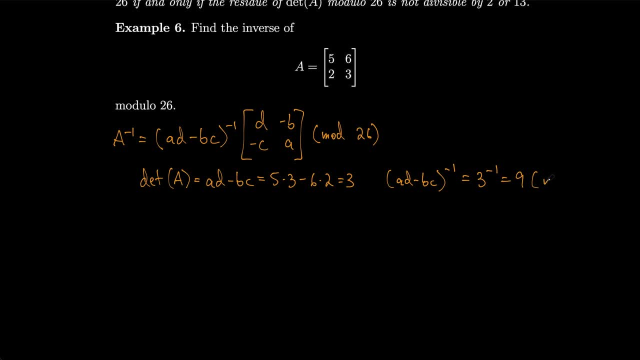 well, that'll be three inverse. well, that'll be three inverse, and we calculated that earlier we saw, and we calculated that earlier we saw, and we calculated that earlier we saw. that that's nine, that that's nine, that that's nine modulo 26.. it's a good thing. we. modulo 26.. it's a good thing we modulo 26.. it's a good thing we calculated that earlier. because calculated that earlier? because calculated that earlier, because otherwise it would have been. otherwise it would have been, otherwise it would have been. you know, we'd have to go through all. 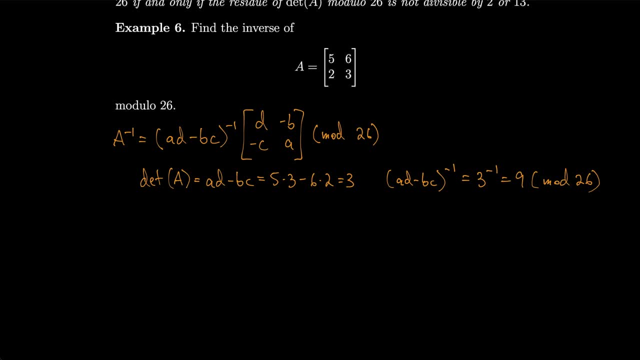 you know, we'd have to go through all you know, we'd have to go through all those numbers from 0 to 25 in order to those numbers from 0 to 25, in order to those numbers from 0 to 25, in order to try to figure out what the inverse was. 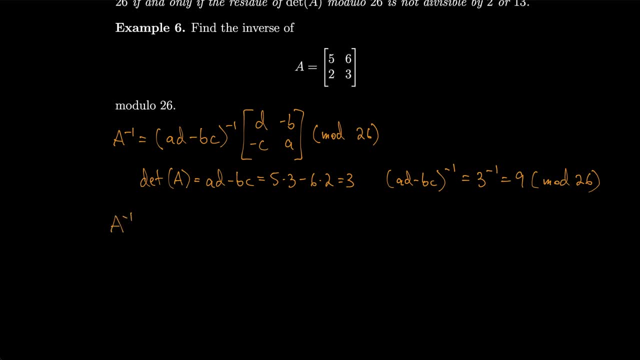 try to figure out what the inverse was. try to figure out what the inverse was, if it even exists. if it even exists. if it even exists, okay. so now we have a inverse is equal to okay. so now we have a inverse is equal to okay. so now we have a inverse is equal to nine. 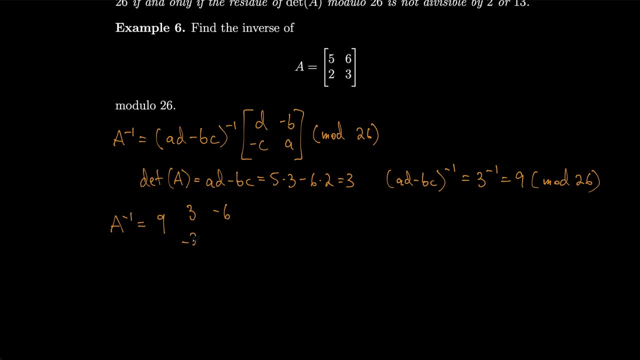 nine nine times three minus six times three minus six times three minus six minus two, five minus two. five minus two, five. just by plugging into our formula now, just by plugging into our formula now, just by plugging into our formula now and multiplying through, we get 27. 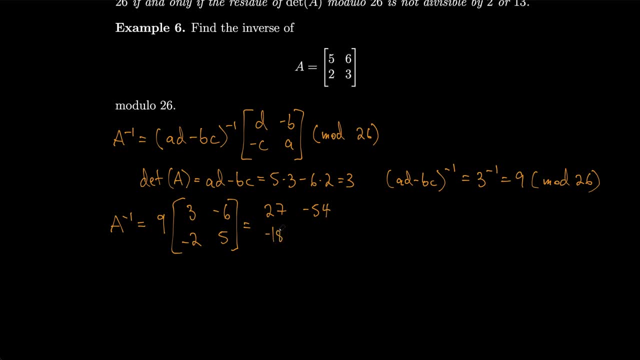 and multiplying through, we get 27, and multiplying through, we get 27 minus 54 minus 18 minus 54 minus 18 minus 54 minus 18, 45, 45, 45. but we have to take this module of 26, so, but we have to take this module of 26, so 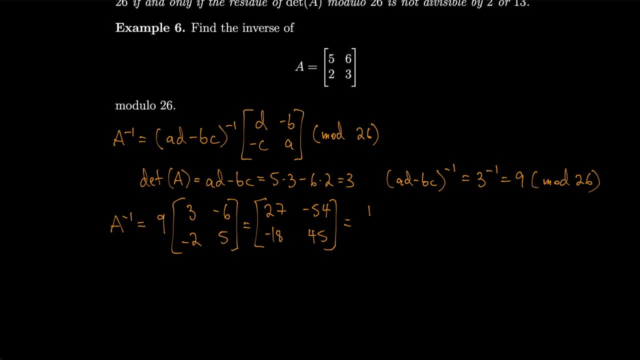 but we have to take this module of 26, so 27, 27, 27 has a remainder of 1 negative, 54 has a. has a remainder of 1 negative. 54 has a. has a remainder of 1 negative. 54 has a remainder of 24. 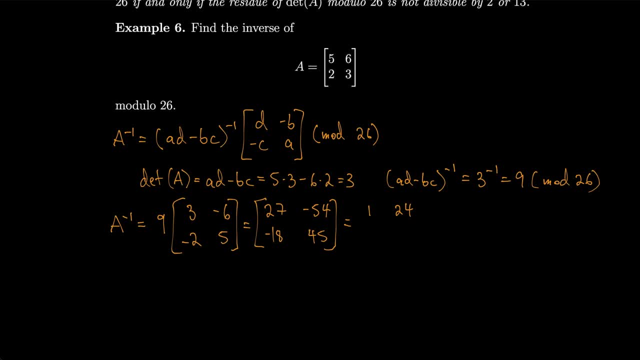 remainder of 24. remainder of 24 over 26. you know everything's out of 26 over 26. you know everything's out of 26 over 26. you know everything's out of 26. and then negative 18 has remainder of 8. 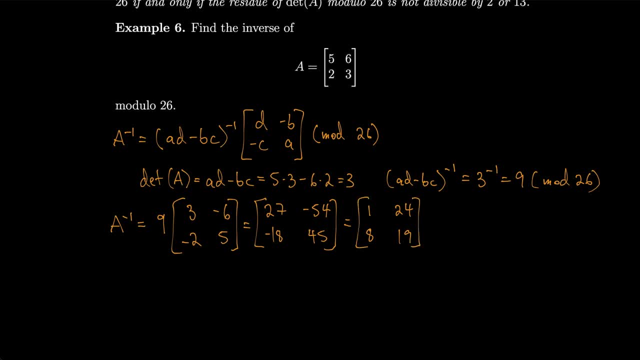 and then negative 18 has remainder of 8, and then negative 18 has remainder of 8, and then, and then, and then 19. 19. 19. so all of that is so, all of that is so. all of that is mod 26. 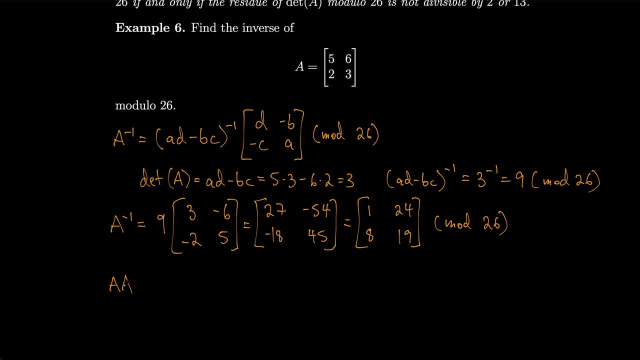 mod 26. mod 26: uh, as a check. we could uh, uh as a check. we could uh, uh, as a check. we could uh, look at a- a inverse. look at a- a inverse. look at a- a inverse, and and, and notice that it'll be five, six. 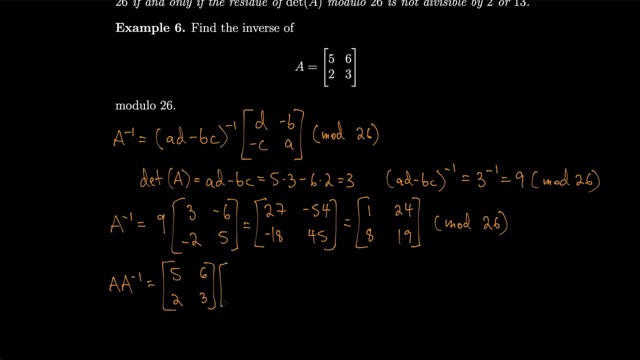 notice that it'll be five, six. notice that it'll be five, six, two, three, two, three, two three times times times 1, 1, 1, 24, 24, 24, 8, 8, 8, 19, 19, 19, so we get 53. 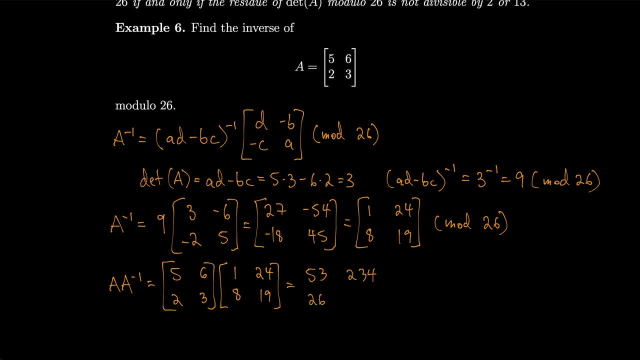 so we get 53. so we get 53. 2, 2, 2, 2, 34, 34, 34, 34, 26, 24, 26, 26, 26, 26, 26, 26, 26, 105, 105, 105 and 234 and 26 are both multiples of 26. 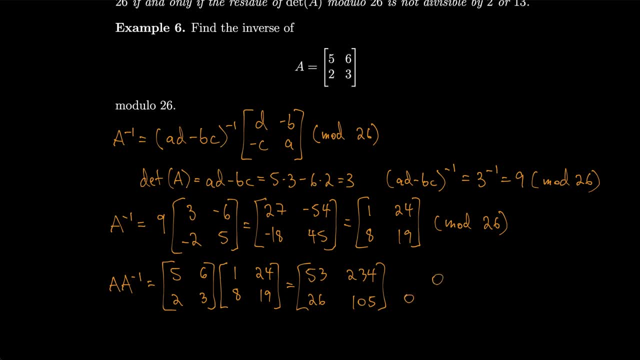 and 234 and 26 are both multiples of 26, and 234 and 26 are both multiples of 26, so those are equal to. so those are equal to. so those are equal to 0 modulo 26 and 53 and 105 have. 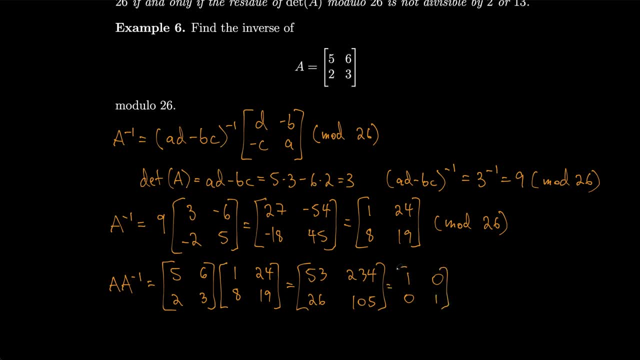 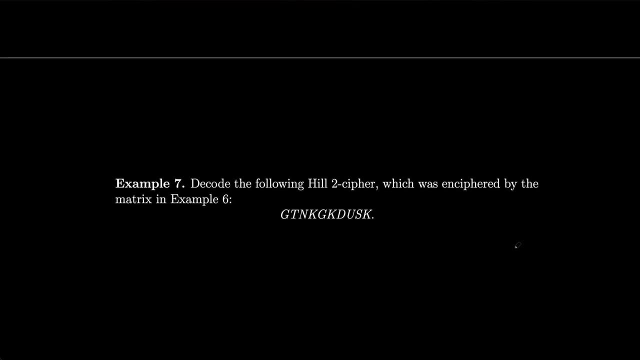 0 modulo 26 and 53 and 105 have 0 modulo 26 and 53 and 105 have remainders of remainders of remainders of 1. so yeah, that's the identity 1. so yeah, that's the identity 1. so yeah, that's the identity mod 26. 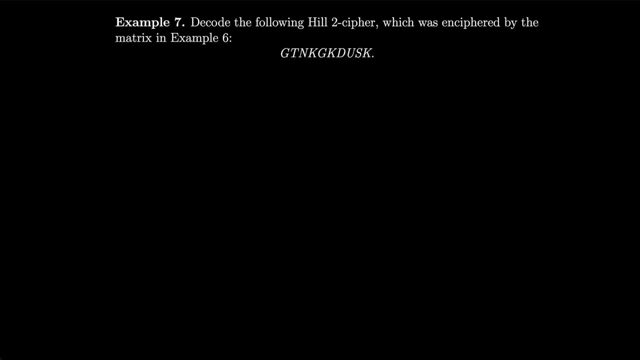 let's decode the following: hill to cipher: let's decode the following: hill to cipher: let's decode the following: hill to cipher: which was in cipher, which was in cipher, which was in cipher, by the matrix in example 6, by the matrix in example 6, by the matrix in example 6. now that we have figured out how to take, 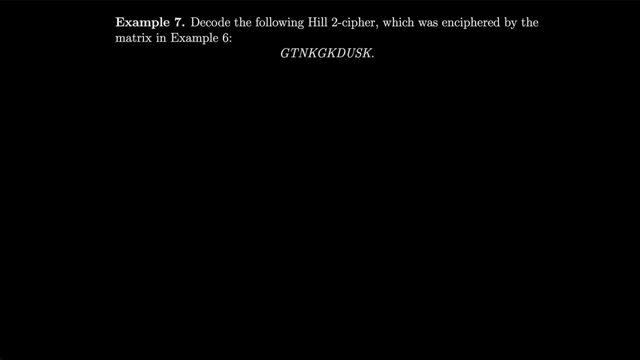 now that we have figured out how to take, now that we have figured out how to take inverses of matrices, inverses of matrices, inverses of matrices with modular arithmetic, we can use those with modular arithmetic, we can use those with modular arithmetic. we can use those inverses. to get back to 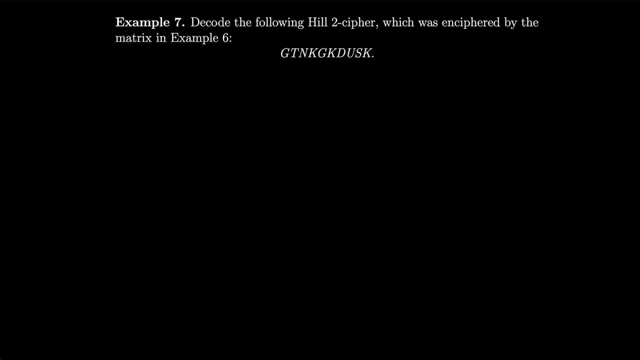 inverses. to get back to inverses. to get back to the uh original um. decoded the uh original um. decoded the uh original um. decoded unenciphered text. so unenciphered text, so unenciphered text. so we, if we're using the matrix in example, 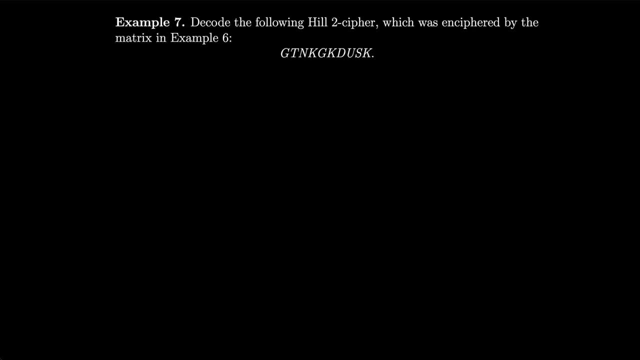 we, if we're using the matrix in example. we, if we're using the matrix in example six, we six, we six. we know that we have the inverse given by. know that we have the inverse given by. know that we have the inverse given by 1: 1. 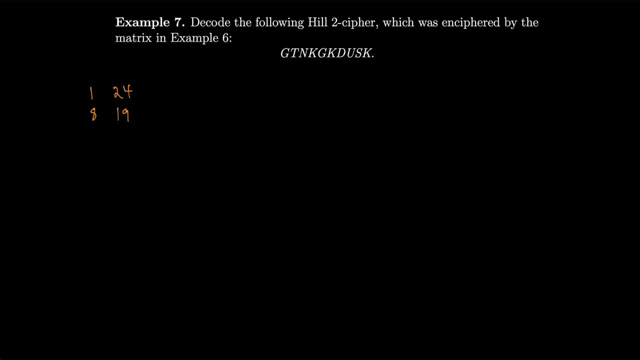 1, 24, 24, 24, 8, 8, 8, 19, 19, 19. so we can take that and multiply it by. so we can take that and multiply it by. so we can take that and multiply it by each of the pairs over here in order to. 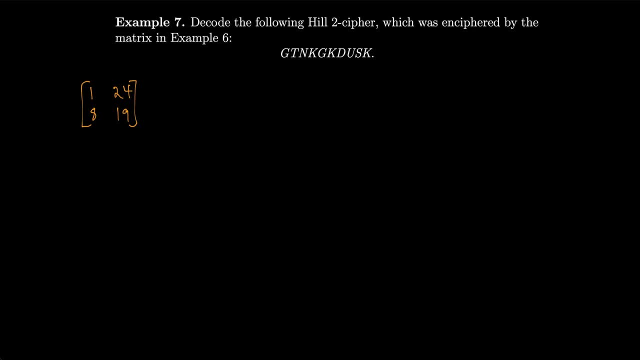 each of the pairs over here, in order to each of the pairs over here, in order to get the get the get the deciphered text. so for g and t, that's deciphered text. so for g and t, that's deciphered text. so for g and t, that's the seventh letter of the alphabet, and 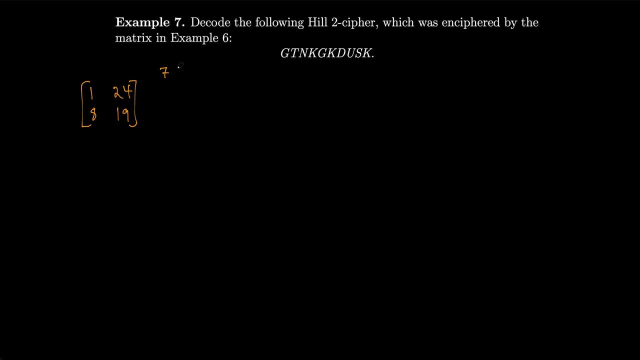 the seventh letter of the alphabet, and the seventh letter of the alphabet and the twent. so we would uh multiply this by, so we would uh multiply this by, so we would uh multiply this by 720, 720, 720, and we would, and we would, and we would get. 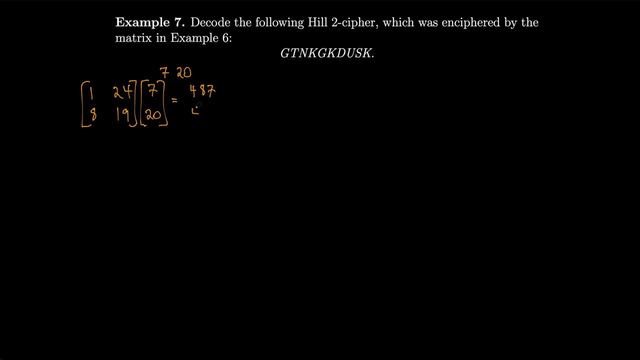 get, get 487, 487, 487, 436, which module 26 is, which module 26 is, which module 26 is 1920.. so that gives us, uh, the letters s and t. so we keep going like this, the uh. so we keep going like this, the uh. 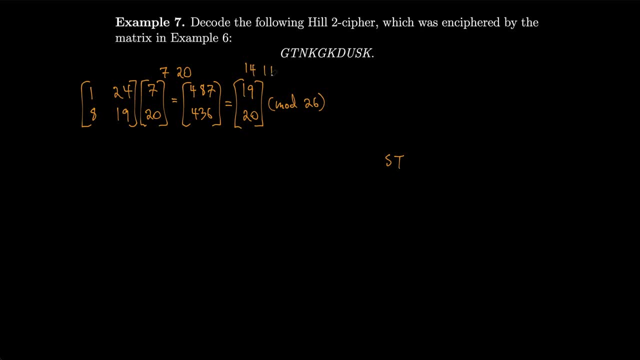 so we keep going like this: the uh, n and k give us 14 and 11, n and k give us 14 and 11, 14 and 11, the G and K give us 7 and 11, then we get 4 and 21, and last we get 19 and 11.. 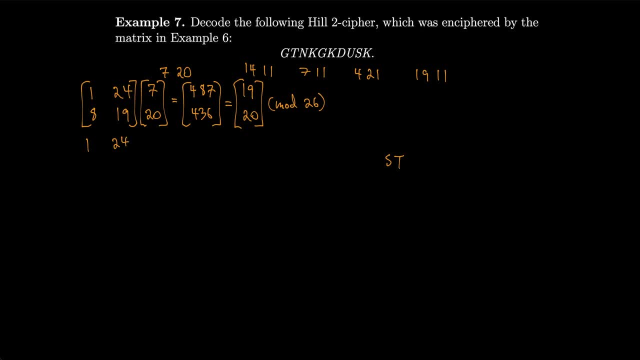 So let's go through each of those pairs. We'll take 1,, 24,, 8,, 19,, multiply it by 14,, 11,, we get 2, 78,, 3, 21,, module 26,, that's 18, 9.. So that gives us Ri. 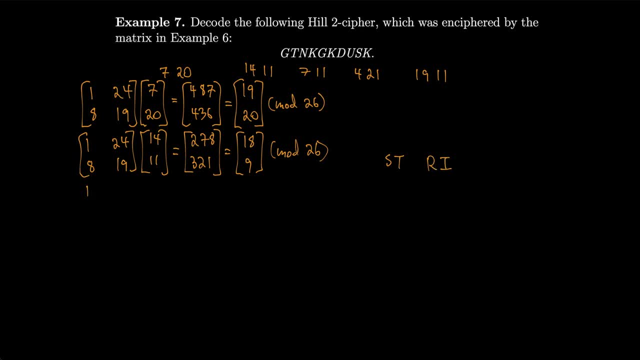 Let's keep going. 1, 24,, 8,, 19, times 7,, 11, gives 2, 71,, 2, 65,, so that's 11, 5,, mod 26,, and that's K. 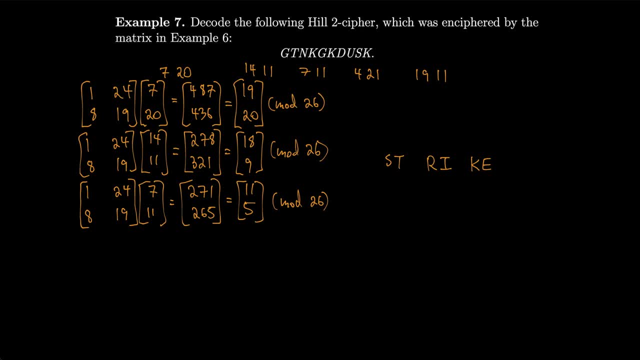 1,, 24,, 8,, 19, times 4,, 21, gives us 5,, 0,, 8,, 4,, 31, module 26, that's 14,, 15. So that gives us N. 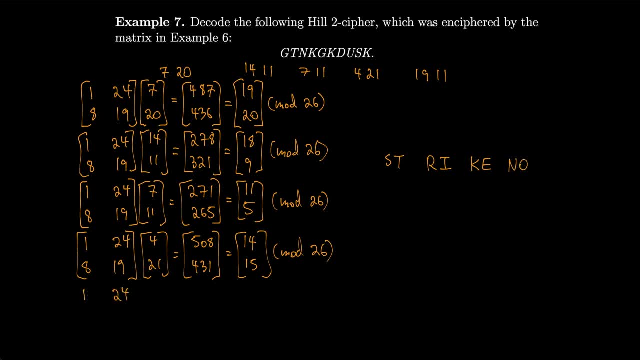 Oh then 1,, 24,, 8,, 19, times 19,, 11, is 2,, 83,, 3,, 61,, which is 23,, 23,, not 26.. So that's W? W. so we have to just kind of read through and try to put the space in ourselves. 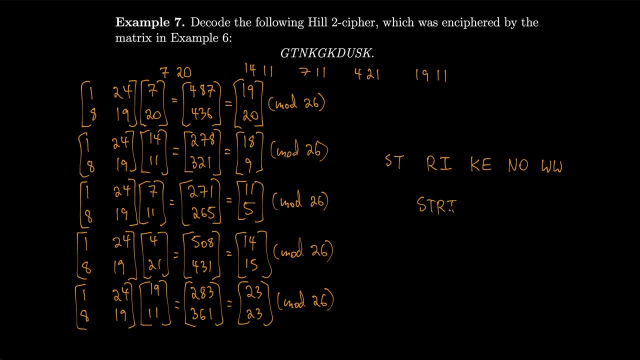 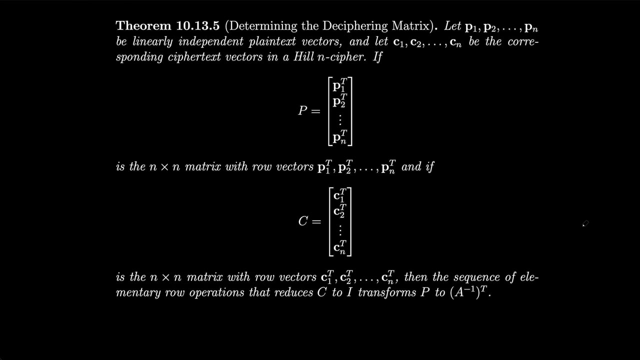 and you can kind of see that it says strike now, because we just won't use that last W. It's superfluous. Add it just to make it an even number of letters In order to determine the deciphering matrix. let P: 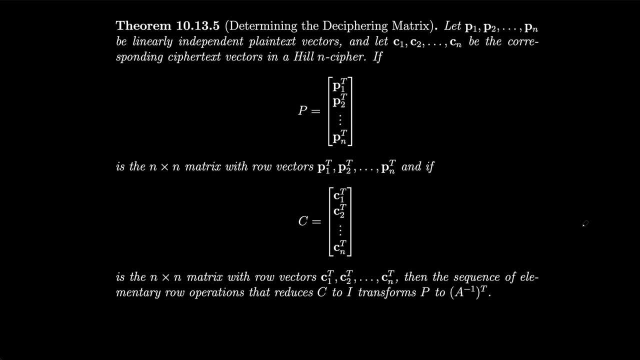 1 through PN be linearly independent plaintext vectors. Let C, 1 through CN be the corresponding ciphertext vectors in a Hill-N cipher, so not necessarily a 2-cypher. If P is given by P1 transpose, P2 transpose and so on, and that's the N-Bion matrix. 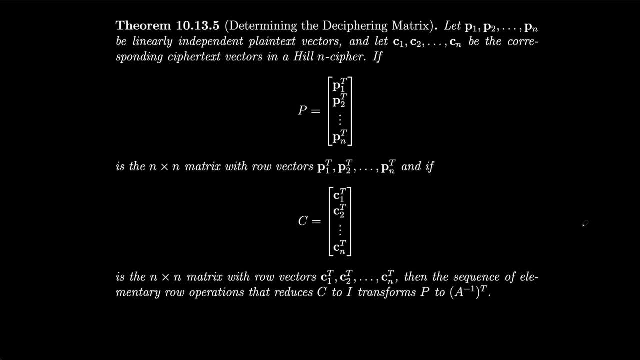 with row vectors: P1- transpose, P2, transpose, et cetera. and if C is given by C1, transpose, C2 transpose, CN transpose, that's the N-Bion matrix. with row vectors: C1 transpose, C2 transpose, et cetera. then the sequence of elementary row operations. 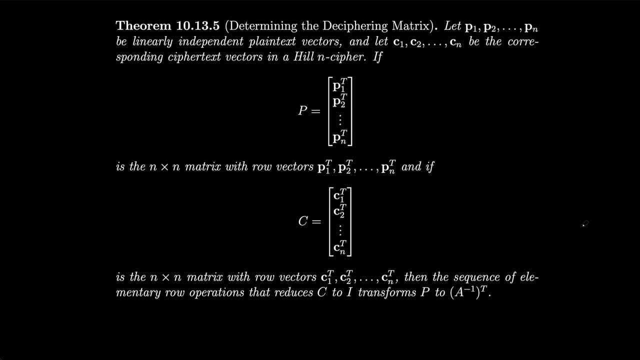 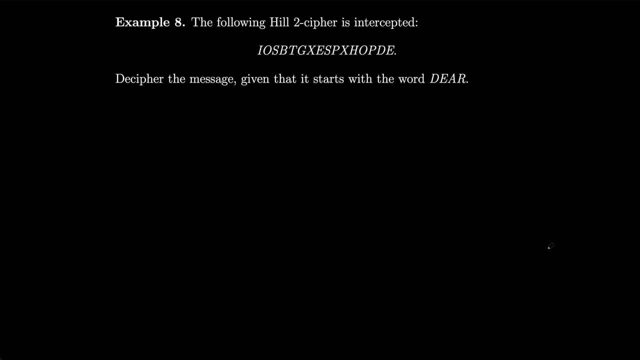 that reduces C to I, transforms P to A inverse transpose. That kind of makes sense that if we're reducing to the identity, of course we're going to get the inverse matrix. So how about we use that? The following Hill-2 cipher is intercepted: 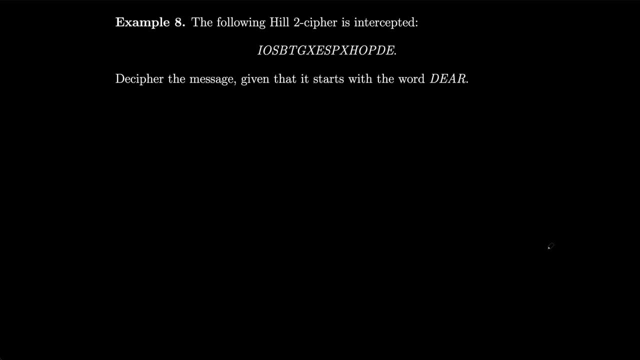 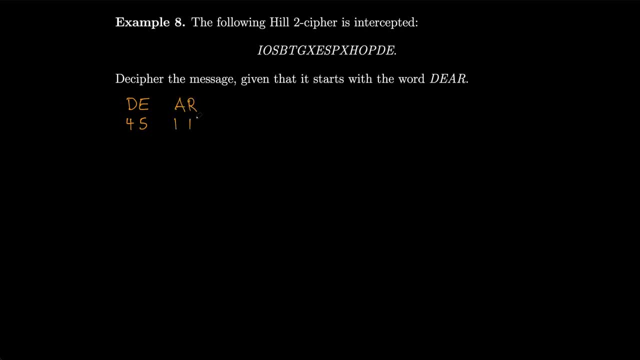 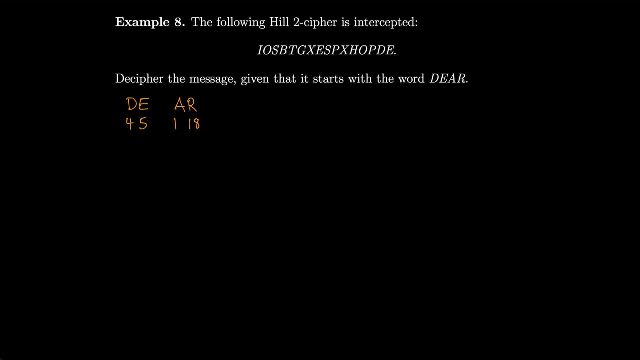 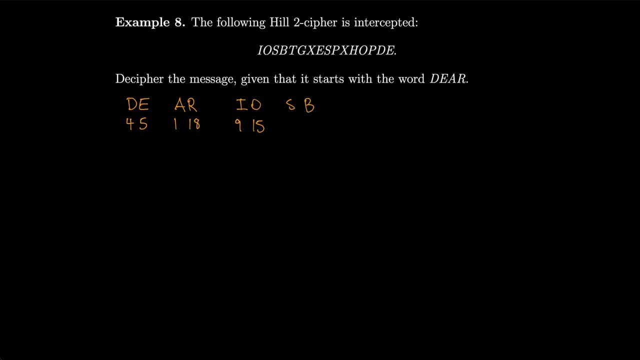 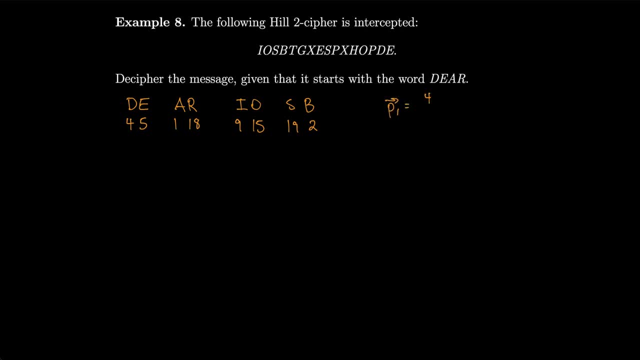 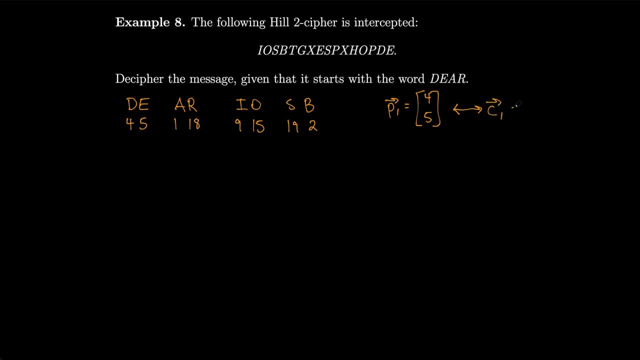 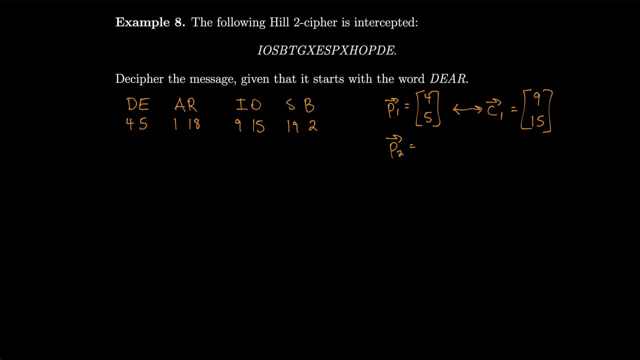 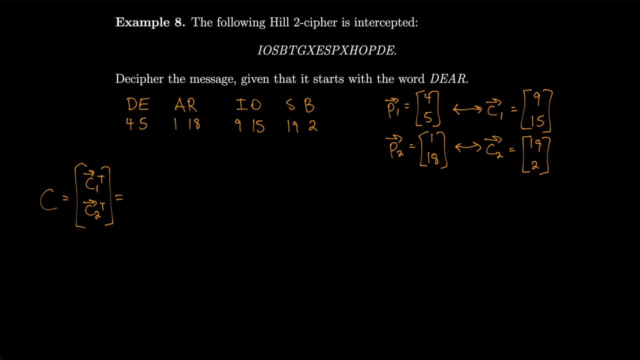 So that'll be 9,, 15,, 19,, 2.. And P is equal to P1 transpose, P2 transpose. So that's 4, 5,, 1. 18.. And let's take 9,, 15,, 19,, 2, and adjoin it with the matrix 4, 5,, 1,, 18,. 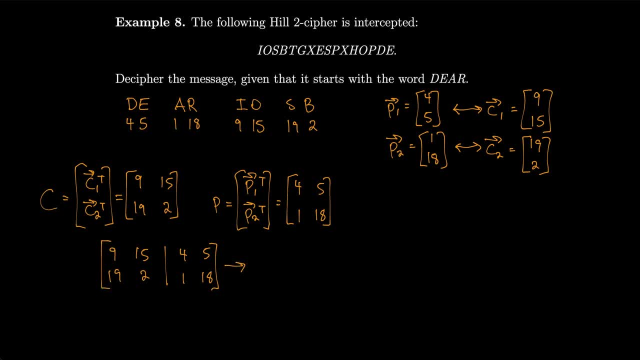 so that we can track what happens as we reduce this matrix to the identity, the matrix on the left. So let's start by multiplying in order to get the leading 1 in the top row. So usually we would divide by 9,. 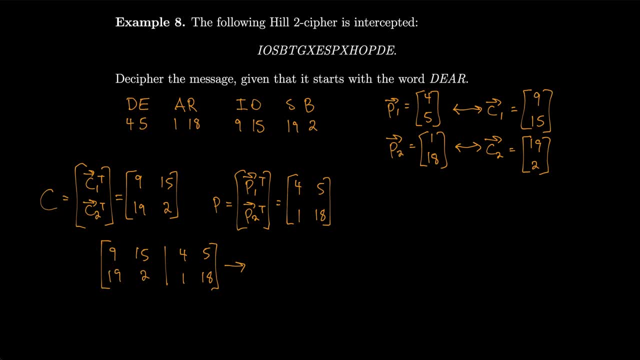 but in this case we have to multiply by 9 inverse mod 26,, which is 3.. Multiplying by that 3 will give us that 1 that we need in order to invert the 9. So multiplying through 3 also gives us. 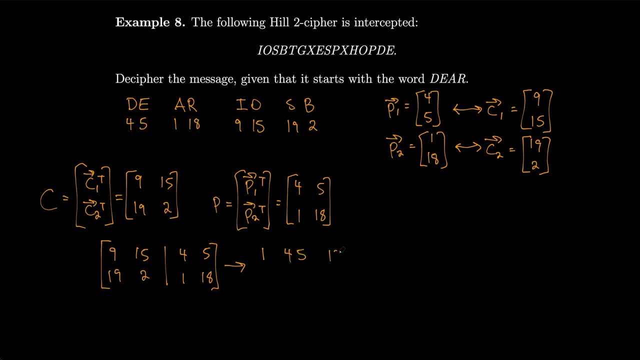 45, and it gives us 12,, and it gives us 15.. So I haven't reduced those yet, but I will, And I'll just keep the second row: 19,, 2,, 1,, 18.. And just showing you the multiplication steps: 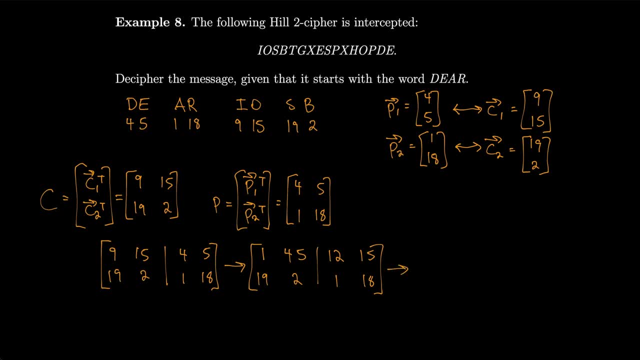 So then we'll reduce 45 mod 26, and 12 and 15, etc. So really just the 45 has to be reduced. So we get 1.. 19,, 12,, 15.. So that's the result of multiplying by 9 inverse, which is 3.. 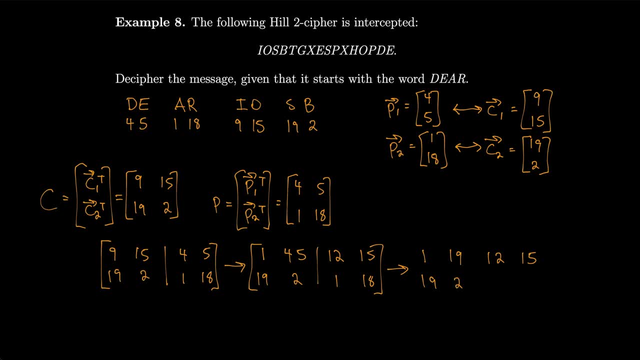 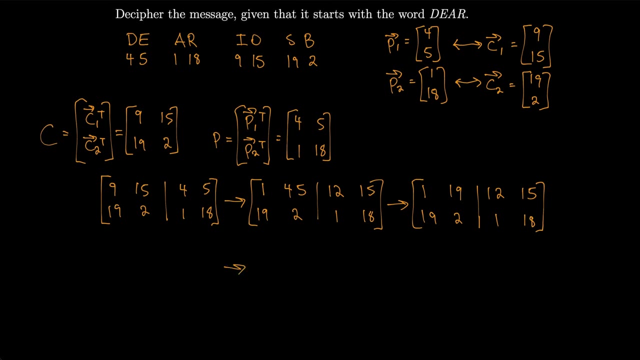 And then taking the result, mod 26.. So we got our leading 1.. It's a little bit trickier because of the modular arithmetic. Let's keep going. So we'll get a 0 underneath by subtracting off 19.. So we'll get a 0 underneath by subtracting off 19.. 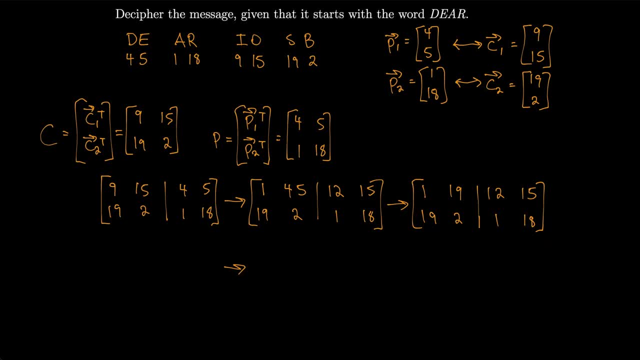 So let's do that. We'll get 1,, 19,, 12,, 15, just by copying the top row On the bottom. we'll get 0 by subtracting 19 times the top row, But we'll also get negative 359,, negative 227, and negative 267.. 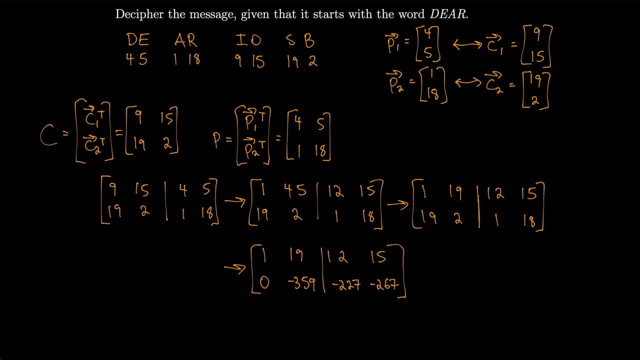 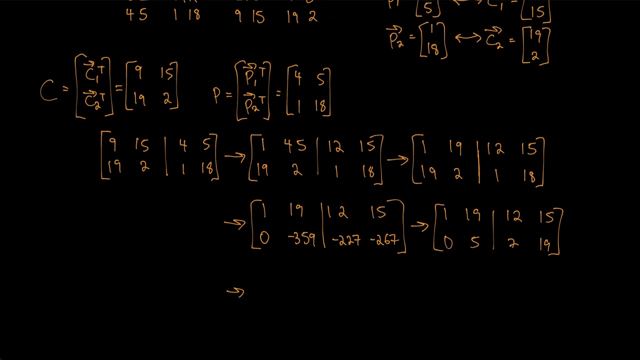 so let's reduce those modulo 26, and we'll keep the top row. 1, 19,, 12,, 15,, 0, 5,, 7,, 19,. keep going. now we have to get a leading one over here. normally we divide by 5,, in this case we 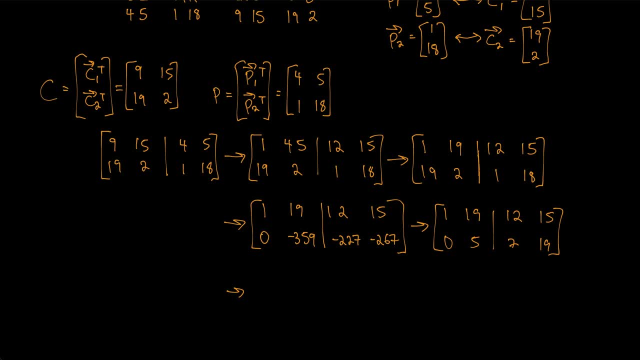 have to multiply by 5, inverse mod 26,, which happens to be 21,. so we'll multiply through everything on the bottom by 21,. so the top row stays the same. bottom gets multiplied by 21,. we get 0,. I'll just take the modulus, because I already know it's the inverse. so give me 1,. 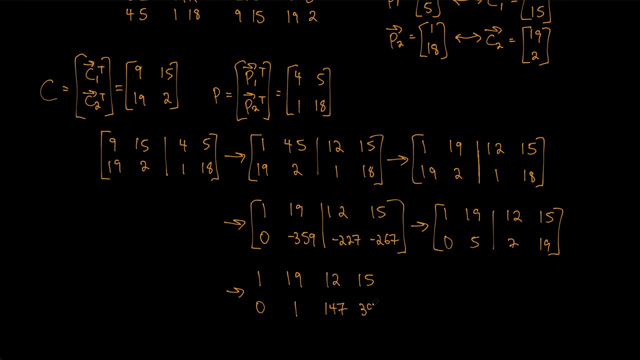 and I'll reduce these in a minute, because I'll get 146,, 7,, 3,, 39, after multiplying, and then I will reduce those, keeping the top the same, so that the bottom becomes 0,, 1,, 17,, 9,. 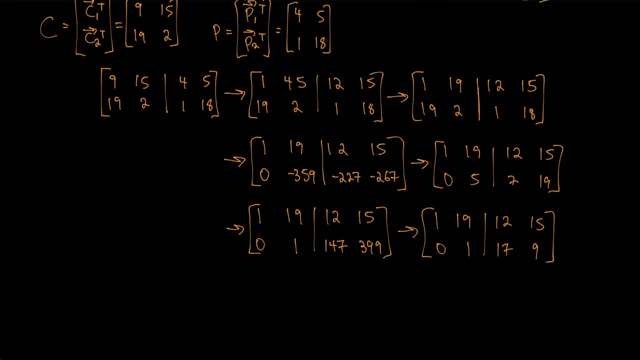 finding that inverse of 5, modulo 26,. not too much fun, by the way, but because you have to go all the way to 21,. but yeah, it's part of the deal. so now on the top, I just subtract 19 times the second row from the first to get a 0, and I'll get negative 311,. 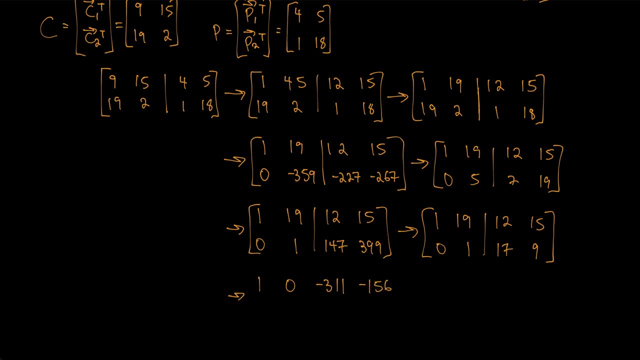 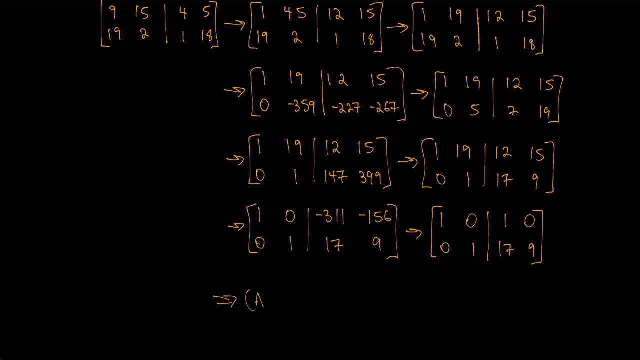 negative 156, on the bottom: 0,, 1,, 17,, 9, and keep going and reduce, we get 1,, 0, 0, 1,, 1,, 0,, 17,, 9, so that gives me my inverse matrix. that means that A inverse transpose must be equal to 1,, 0,, 17,, 9,. 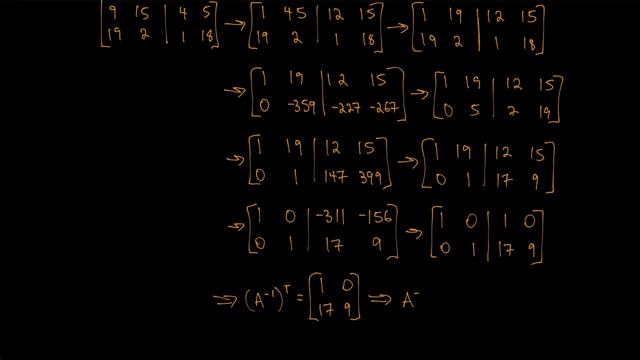 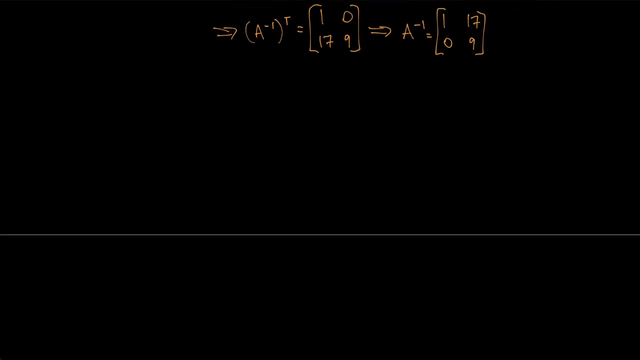 and therefore I just have to take the transpose and I'll get A inverse, so that'll help me decipher this code. so 1, 17,, 0, 9.. So how about we use that? we have I, O, S, B, T, G, X, E, S, P, X, H, O, P, D, E. 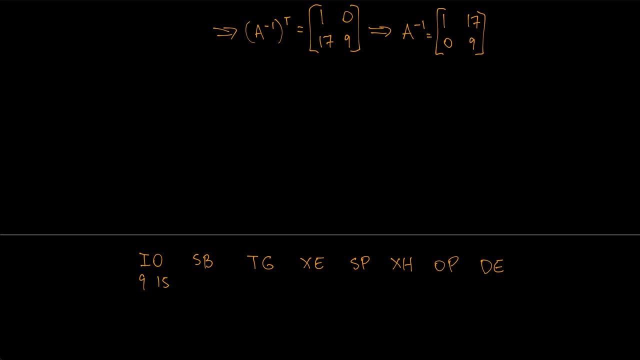 so that was 9, 15,, 19,, 2, 27,, 24,, 5,, 19,, 16,, 24,, 8,, 15,, 16, and 4, 5.. So we'll take our matrix 1, 17,, 0, 9,. 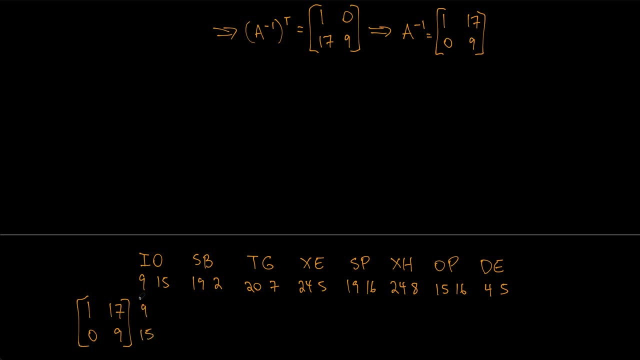 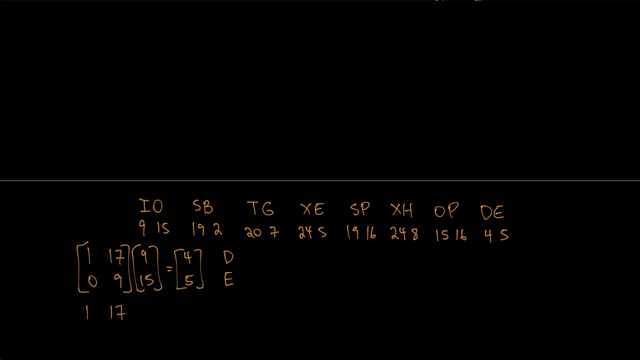 multiply it by I, O, which is 9,, 15,, to decipher it, and get 4,, 5,, which is D, E, as we wanted, because the first word should be dear. so then 1,, 17,, 0,, 9, times S, B, which is 19,, 2, gives us 1,, 18,. 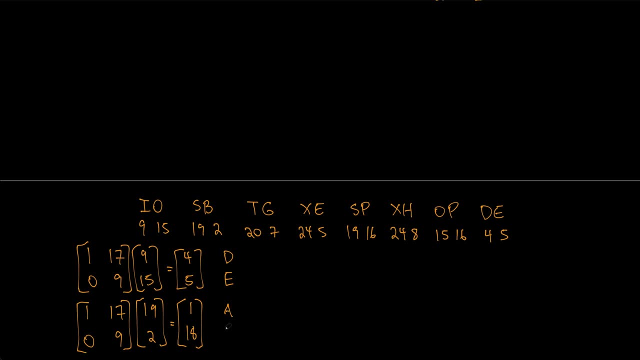 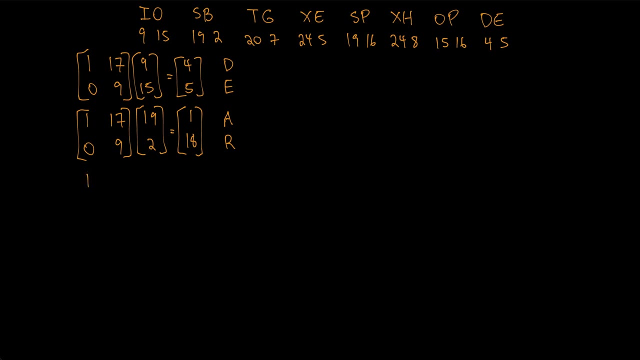 and we get that A R that we wanted. So now the interesting part is the rest of the message, because we don't know what that is yet. so 1, 17,, 0, 9, times 27, gives us 9, 11, so that's I K. 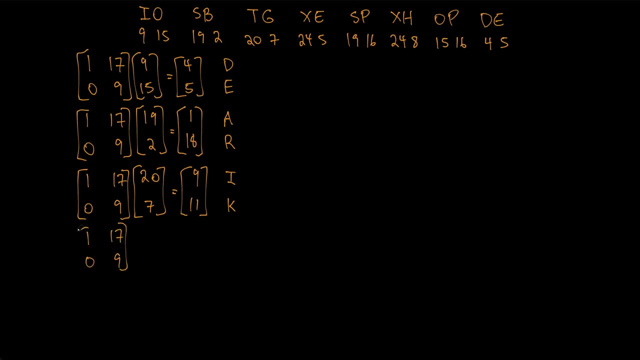 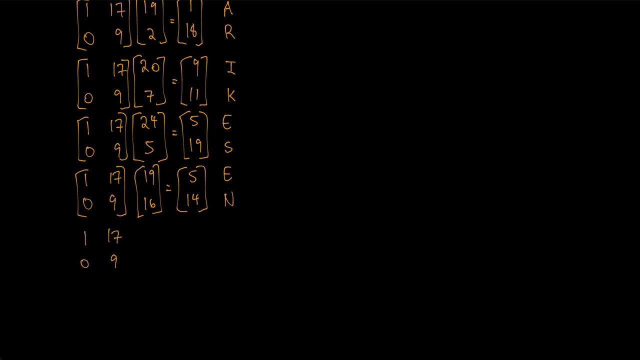 Then 11709 times 245 gives 519,, which is ES11709 times 119,16 is 514.. So that's EN, And then 11709 times 248 is 420, which is the total number of units that will be. is the ideas that themutants of the 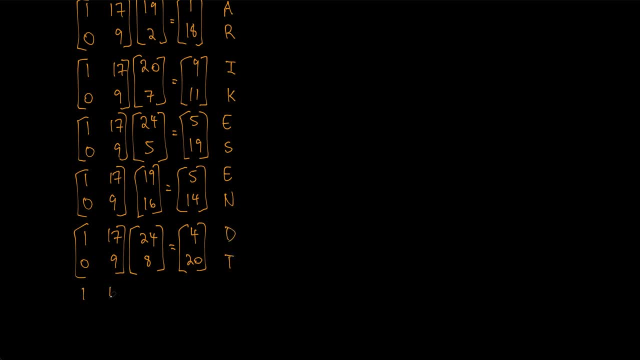 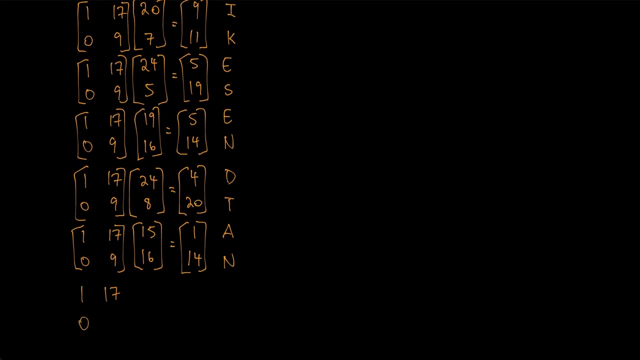 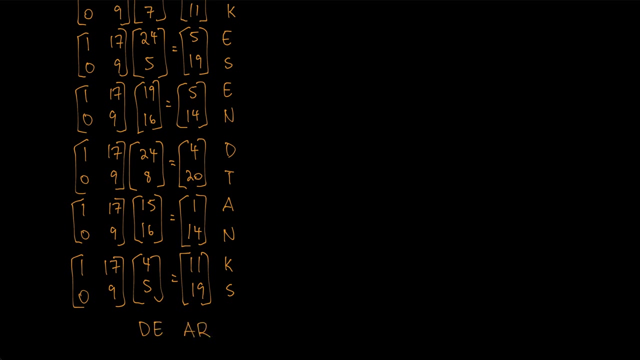 is D, T, then 1, 17, 0, 9 times 15, 16 is 1, 14, which is a n. and last but not least, we have 1, 17, 0, 9 times 4, 5, giving us 11, 19, and that's K? S. so all together we have D, E, A, R, I, K, E S E N D.